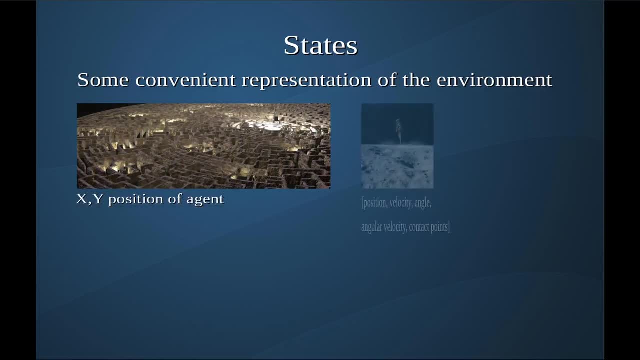 maze. The state can be more abstract, like in the case of the lunar lander, where the state is an array of continuous numbers that describe the position of the lander, the velocity and angular velocity, as well as which legs are in contact with the ground. The main idea. 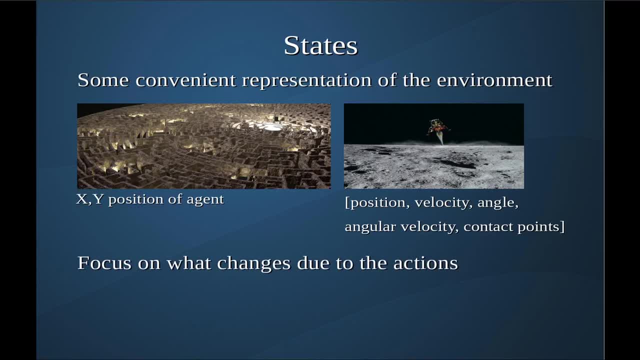 is that the state describes exactly what about. the environment is changing at each time step. The rules that govern how the states change are called the dynamics of the environment. The actions are a little simpler to understand In the case of a maze-running robot. the actions 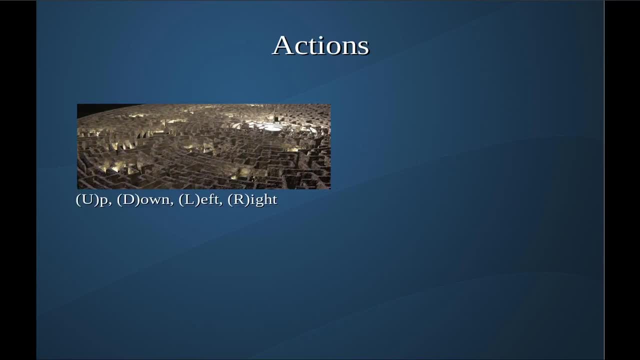 would be just move up, down, left and right, Pretty straightforward. In the case of the lunar lander, the actions consist of doing nothing, firing the main engine and moving in, firing the left engine and firing the right engine. 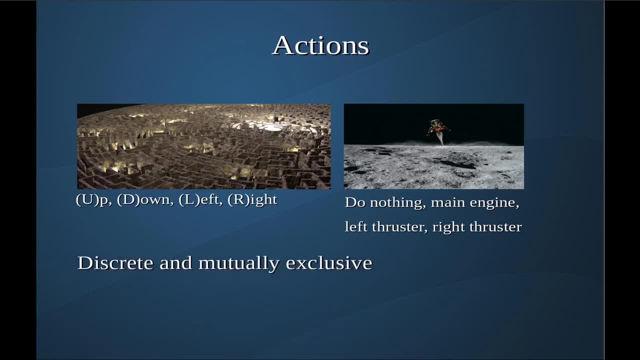 In both these cases, the actions are discrete, meaning they're either one or the other. You can't simultaneously not fire the engine and fire the right thruster, for instance. This doesn't have to be the case, though. Actions can in fact be continuous, and there are numerous. 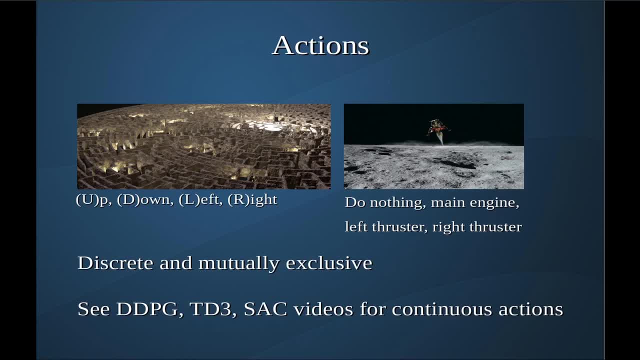 videos on this channel dealing with continuous action spaces. Check out my videos on soft actor critic, deep deterministic policy gradients and twin-delayed deep deterministic policy gradients. From the agent's perspective, it's seeing some set of states and trying to decide what. 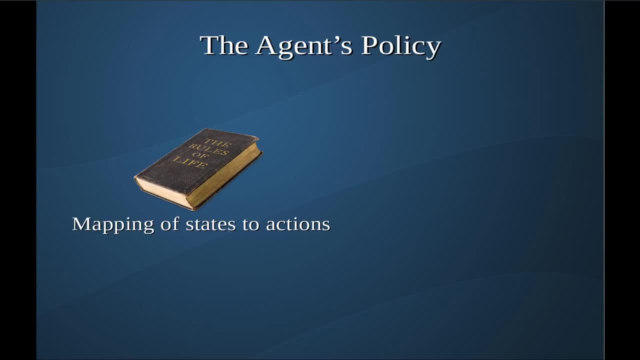 to do. How is our agent to decide? The answer is something called the agent's policy. A policy is a mathematical function that takes states as inputs and returns probabilities as output. In particular, the policy assigns some probability to each action in the action. 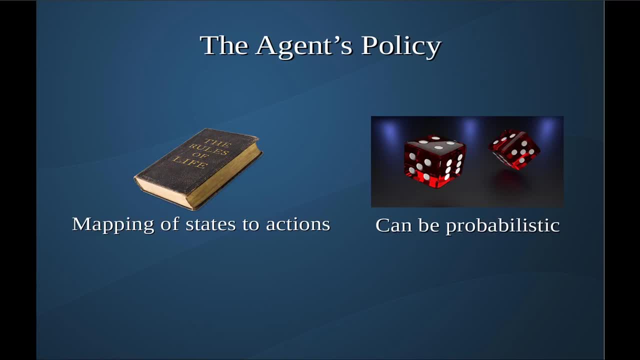 space for each state. It can be deterministic, meaning the probability of selecting one of the actions as 1 and the others as 0, but in general the probability of selecting one of the actions as 0 or 1but is much less than 0.. The policy is typically denoted by the 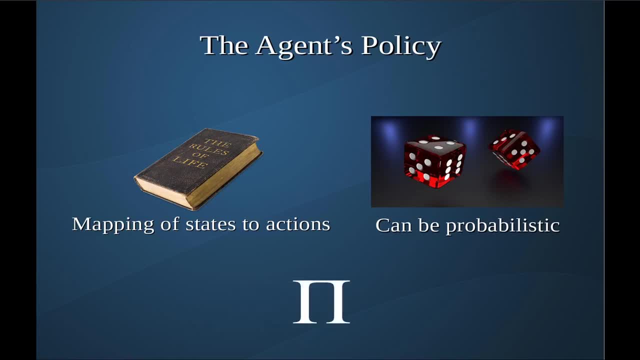 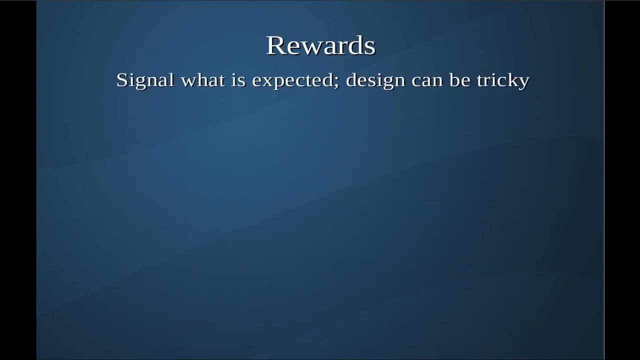 Greek letter Pi and learning to beat the environment is, then, a matter of finding the policy Pi that maximizes the total return over time by increasing the chances of selecting the best actions and reducing the chances of selecting the wrong actions. The rewards tells the agent exactly what is expected of it. The rewards can be either: 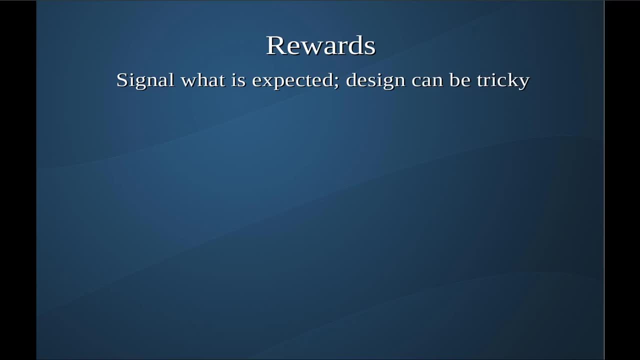 positive or negative, and the design of rewards is a tricky issue. Let's take the maze running robot. If we give it a positive reward for exiting the maze and no other reward, what is the consequence of that? The consequence is that the agent has no motivation. 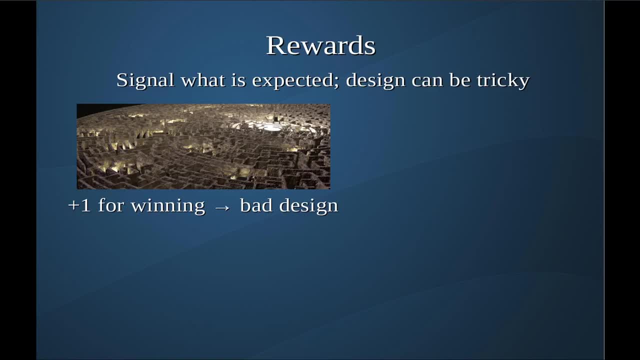 to solve the maze quickly. It gets the same reward if it takes the minimum number of steps or if it takes 100 times that number. We typically want to solve the maze as quickly as possible, so this simple reward scheme fails In this example. we have to give a penalty. 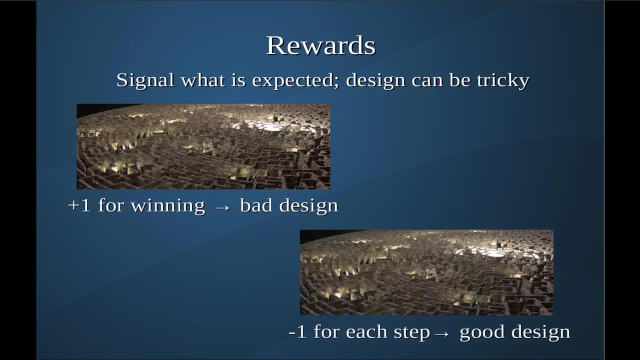 or reward of minus one for each step and a reward of zero for exiting the maze, Then the agent has a strong motivation to solve the maze in as few steps as possible. This is because the agent will be trying to maximize the negative reward, meaning get it as close to zero as possible. 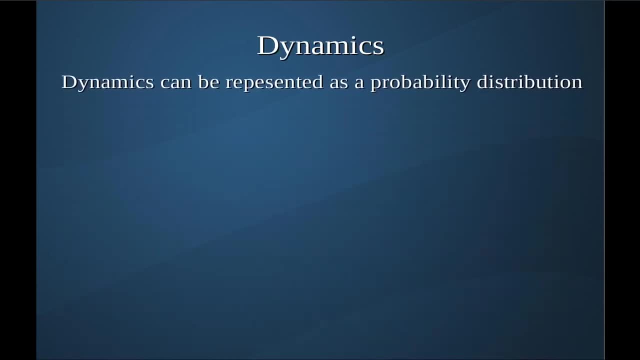 So now that we have our basic definitions out of the way, we can start to think through the mathematics of the reinforcement learning problem From the agent's perspective. it has no idea how its actions affect the environment, so we have to use a probability distribution. 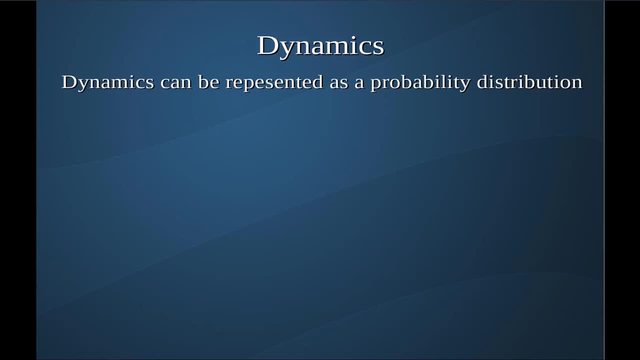 to describe the dynamics. This probability distribution is denoted P of S prime in R given S and A, which just reads as the probability of ending up in state S prime and receiving reward. R, given we are in state S and take action. A. In general, we won't know the value for this. 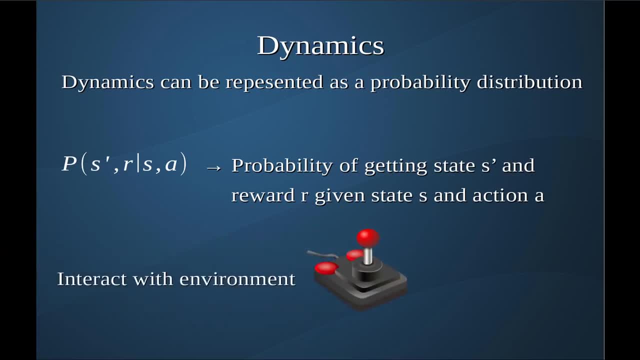 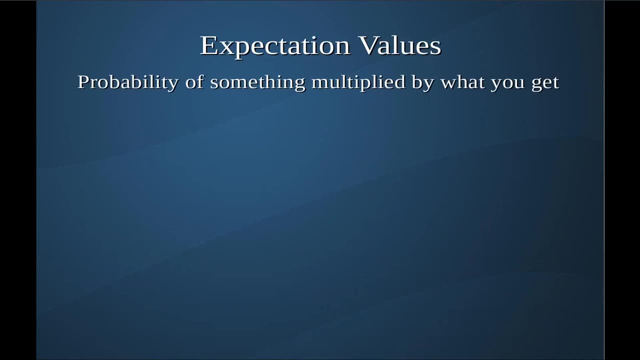 until we interact with the environment, and that's really part of solving reinforcement learning. Since we're dealing with probabilities, we have to start thinking in terms of expectation values. In general, the expectation value is calculated by taking into account all possible outcomes and multiplying the probability of that outcome. 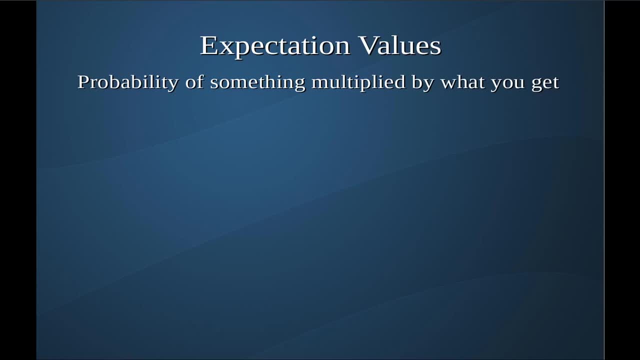 by what you receive in that outcome. So in our Markov framework the expected reward for a state and action pair is given by the expectation value of that reward, which is the sum over all possible rewards, the outcomes multiplied by the sum over the probabilities. 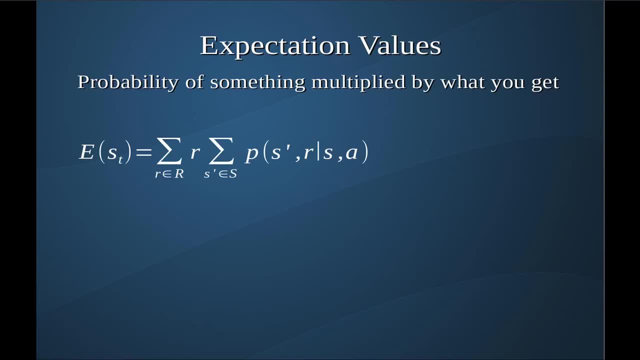 of ending up in all possible resulting states. For a simple example, let's consider a simple coin toss game. If we flip a coin and it comes up heads, you get one point. If it comes up tails, you get minus one point. 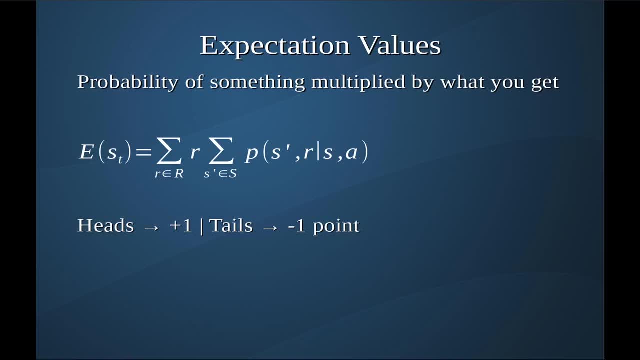 If we flip the coin two times, what is the expected number of points? It's the probability of getting heads multiplied by the reward for getting heads, plus the probability of getting tails multiplied by the reward for getting tails. So it's 0.5 times one plus 0.5 times negative one. 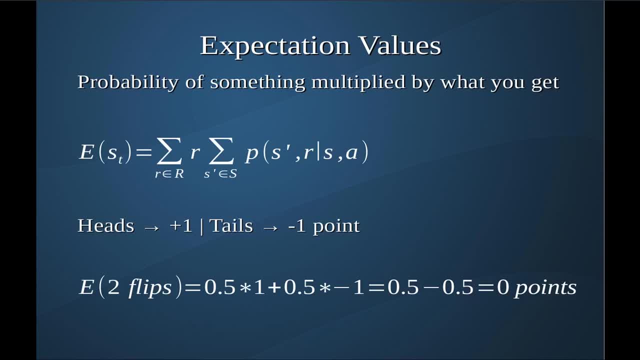 This gives an expected reward of zero points, which is what you would intuitively expect. This is a trivial example, but I hope it illustrates the point. We have to consider all possible outcomes, their probabilities and what we would expect to receive in each of those outcomes. 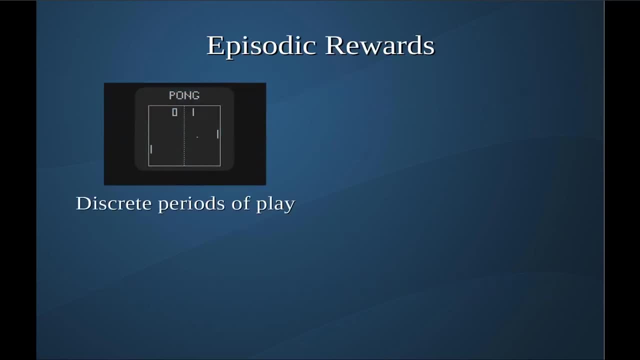 When we go to put theory in practice. we're going to look at. When we go to put theory in practice, we're going to be doing it in systems that are what we call episodic. This means that the agent has some starting state. 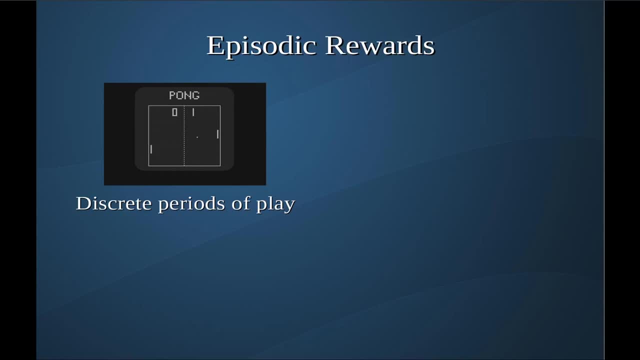 and there is some terminal state that causes the gameplay to end. Of course, we can start over again with a new episode, but the agent takes no actions in this terminal step and thus no future rewards follow. In this case, we're dealing with not just individual rewards. 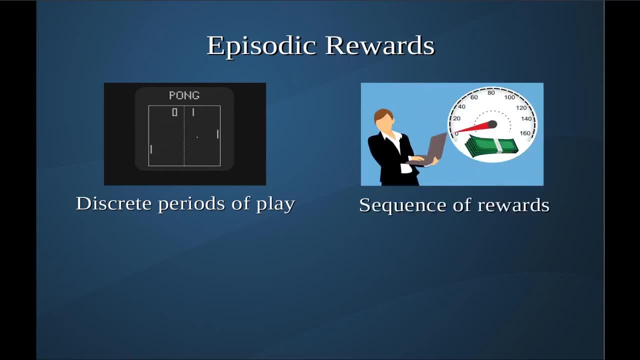 but with the sequence of rewards over the course of that episode. We call the cumulative reward the return, and it's usually denoted by the letter G. Now, this discussion is for games that are broken into episodes, but it would be nice if we could use the same mathematics. 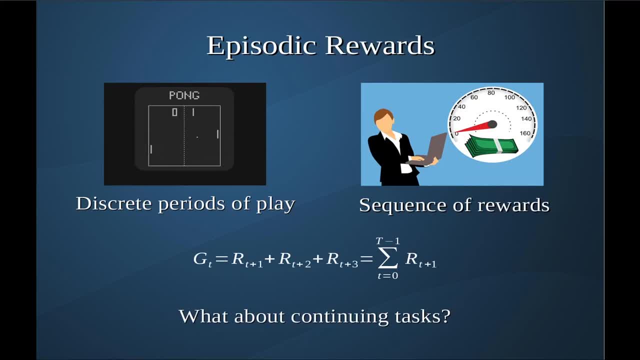 for tasks that don't have a natural end. If we have a game that goes on and on, then the total sum of rewards will approach infinity. It's absurd to talk about maximizing total rewards in an environment where you can expect an infinite reward. 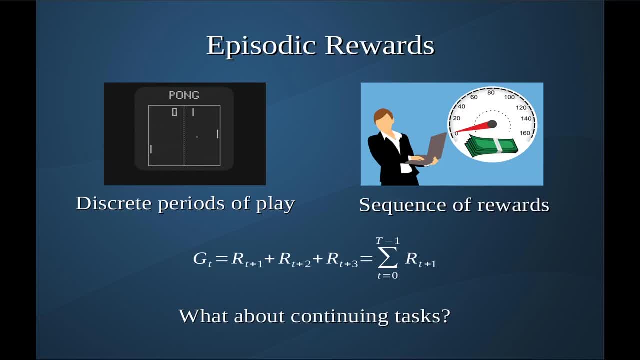 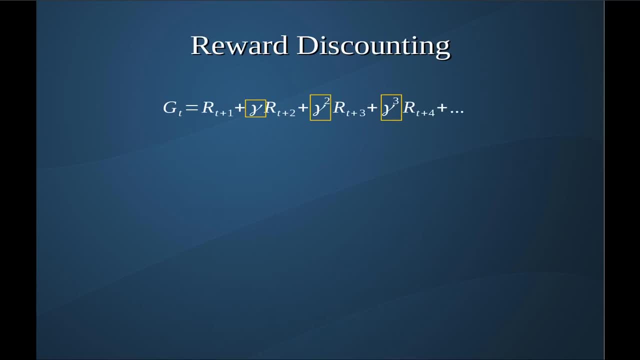 so we have to do a little modification to our expression for the returns. We need to introduce the concept of discounting. We're going to reduce the contribution of each reward to the sum based on how far away we are from the reward and how far away in time it is from our current time step. 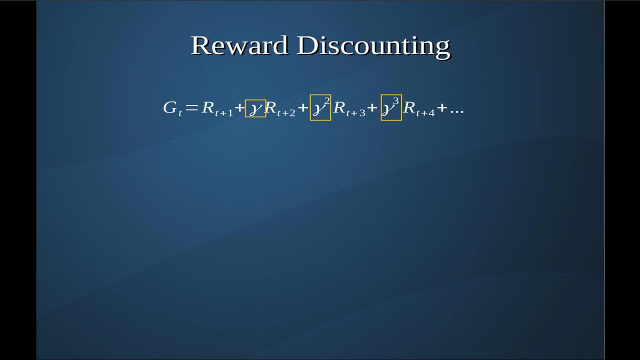 We're going to use a power law to describe this reduction, so that the reward gets reduced by some additional power of a new hyperparameter we'll denote as gamma. Gamma is between zero and one, so each time we increase the power, the contribution is reduced. 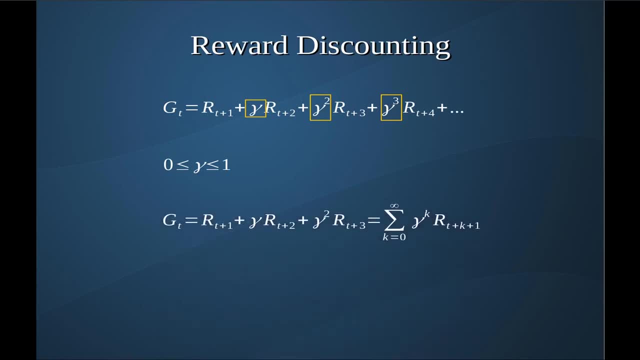 If we introduce gamma into the expression for the return at time step t, we get that the return is just the sum over k of gamma to the k multiplied by the rewards at time t plus one plus k. Besides being a trick to make sure we can use, 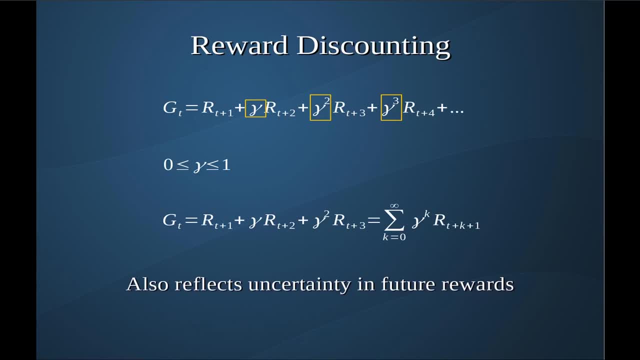 the same mathematics for episodic and continuing tasks. discounting has a reasonable basis in first principles. Since our state transitions are defined in terms of unknown probabilities, we can't really say how certain each of those rewards were, States that we encounter further out in time. 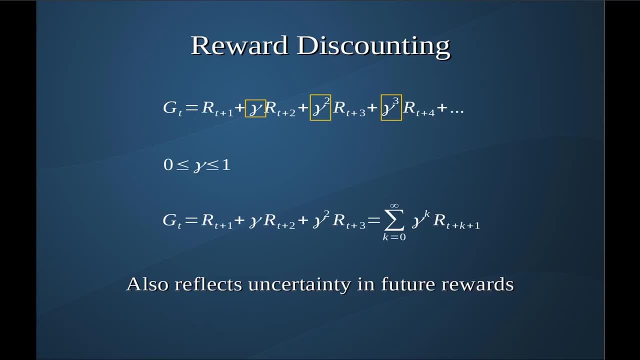 become less and less certain, and so the rewards for reaching those states are also less and less certain. Thus, we shouldn't weight them as much as the reward we just received. If you've been following along carefully, something may not quite add up here. 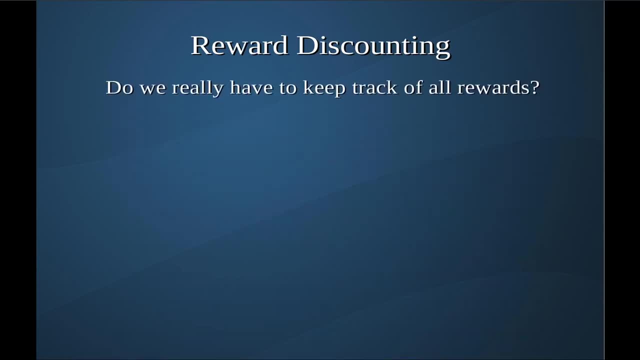 All this math is for systems with the Markov property, which means that they depend only on the previous state in action. so why do we want to keep track of the entire history of rewards received? Well, it turns out that we don't have to. 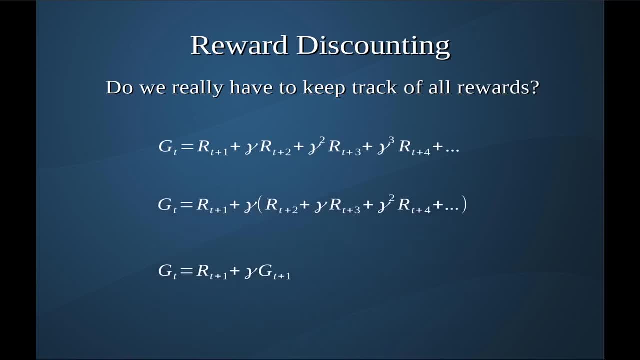 If you do some factoring in the expression for the return at time step t, you find that the return at time t is just the sum of the reward at time t plus one and the discounted return for the t plus one time step- a recursive relationship between returns at each time step. It's more consistent with the 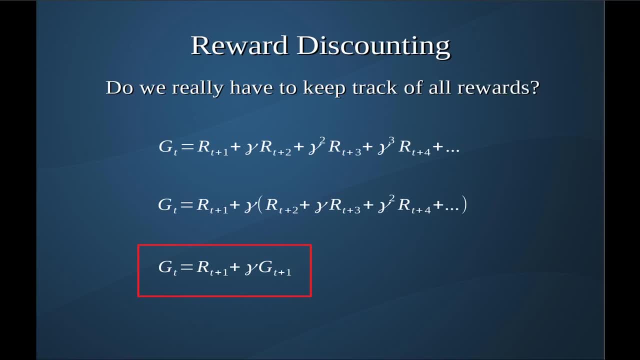 principles of the Markov decision process, where we're just concerned with successive time steps. Now that we know exactly what the agent wants to maximize the total returns and then function for how it's going to act, the policy- we can actually start to make useful mathematical. 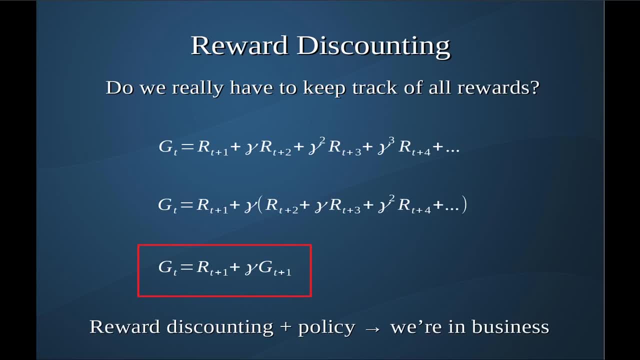 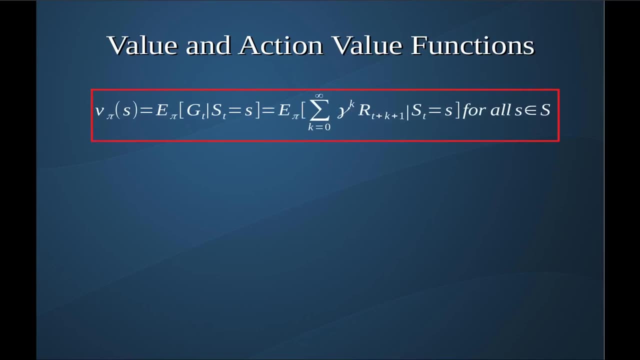 predictions. One quantity of particular interest is called the value function. It depends on the agent's policy pi and the current state of the environment and gives us the expectation value of the agent's returns starting from time t and state s, assuming it follows the policy pi. 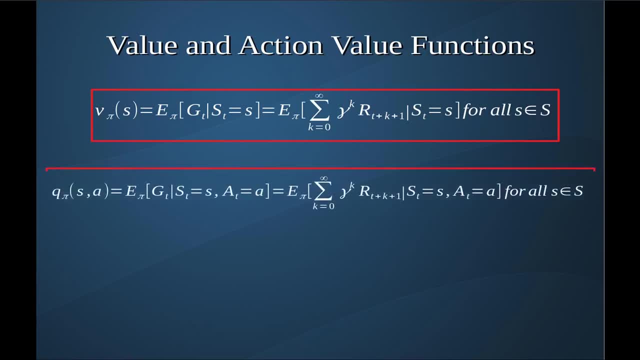 There's a comparable function for the value of state and action pairs which tells us the value of taking action a and state s and then following the policy pi afterwards. It's called the action value function and it's represented by the letter q. So how are these values calculated in practice? 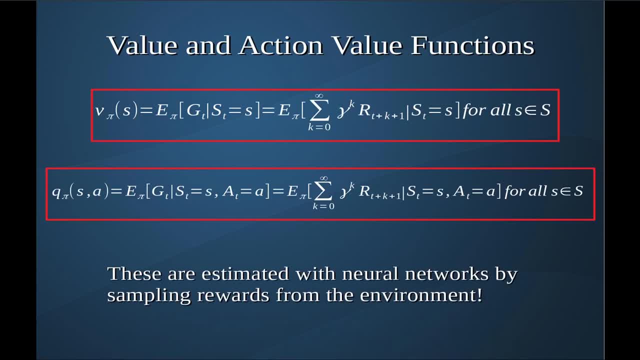 Well, in reality we don't solve these equations, we estimate them. We can use neural networks to approximate the value or action value function, because neural networks are universal function approximators. We sample rewards from the environment and use those to update the weights of our network to improve our estimate for the. 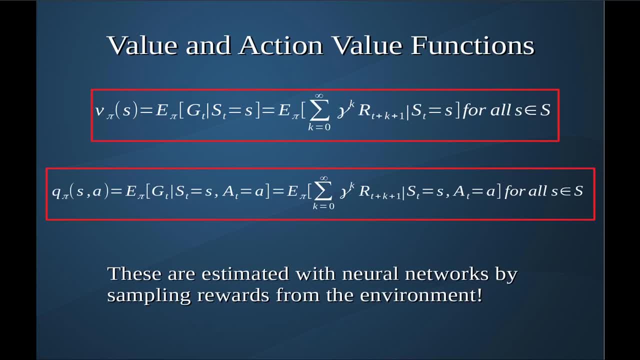 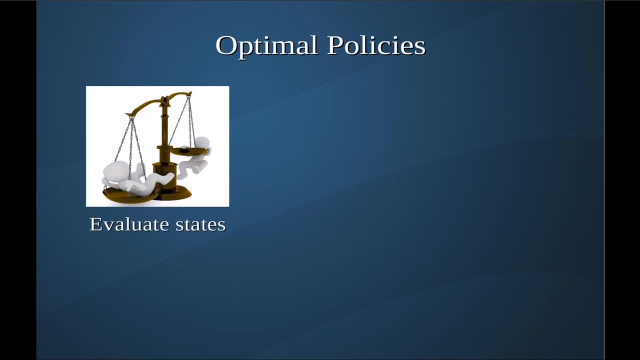 value or action value function. Estimating the value function is important because it tells us the value of the current state and the value of any other state the agent may encounter. Solving the reinforcement learning problem then becomes an issue of constructing a policy that allows the 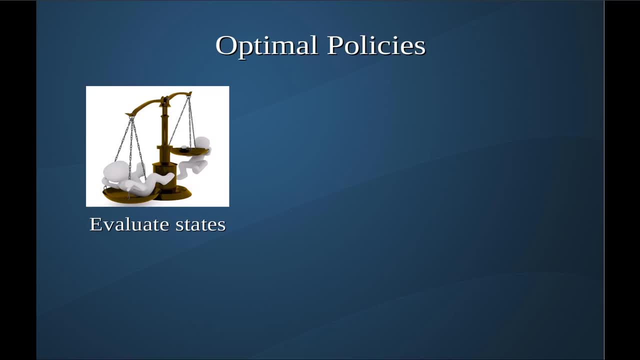 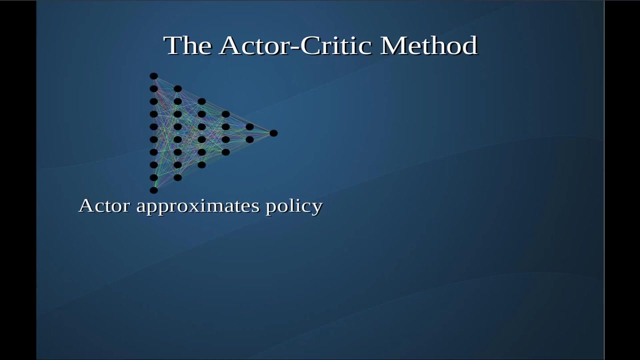 agent to seek out the most profitable state. One way for us to find this optimal is by looking at relations and graphs. The policy which we'll be taking a look at is called a probability distribution over the set of actions, where we take a state as input and output a. 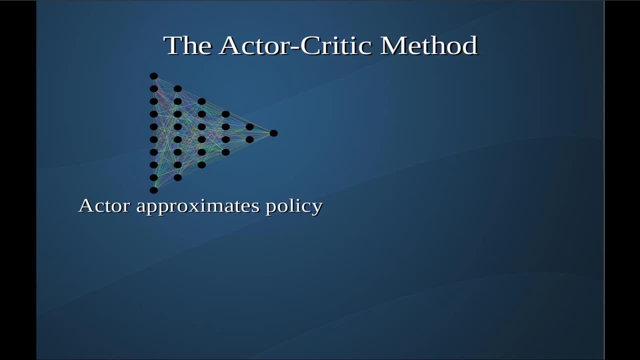 probability of selecting each action. The other network, called the critic, is used to approximate the value function. The critic acts just like any other critic, telling the actor how good each action is based on whether or not the resulting state is valuable. The two networks work together. 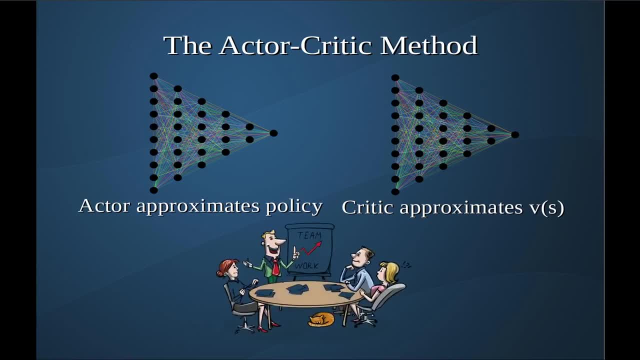 to find out how best to act in the environment. The actor selects actions, the critic evaluates the states and then the result is compared to the rewards from the environment. Over time, the critic becomes more accurate at estimating the values of states, which allows the actor to. 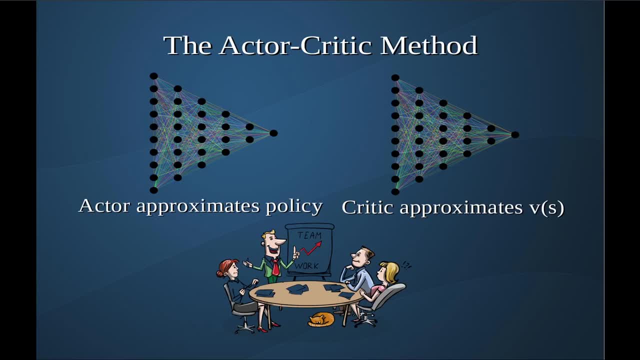 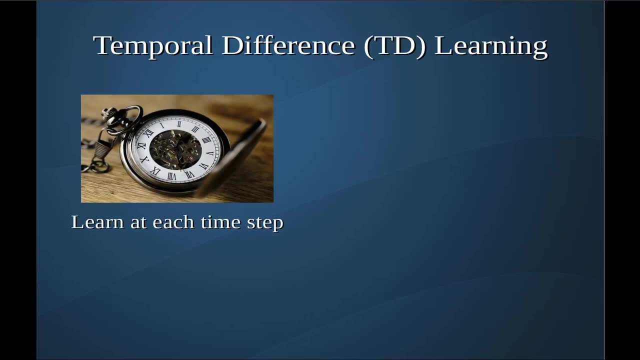 select the actions that lead to those states. From a practical perspective, we're going to be updating the weights of our deep neural network at each time step, because actor-critic methods belong to a class of algorithms called temporal difference learning. This is just a fancy way of. 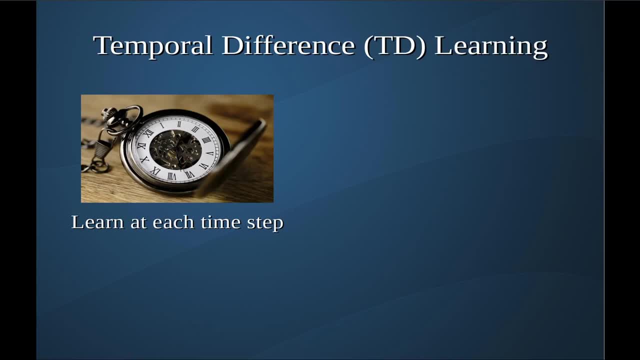 saying that we're going to be estimating the difference in values of successive states, meaning states that are one time step apart, hence temporal difference. Just like with any deep learning problem, we're going to be calculating cost functions. In particular, we're going to have two cost functions: one for updating our critic and 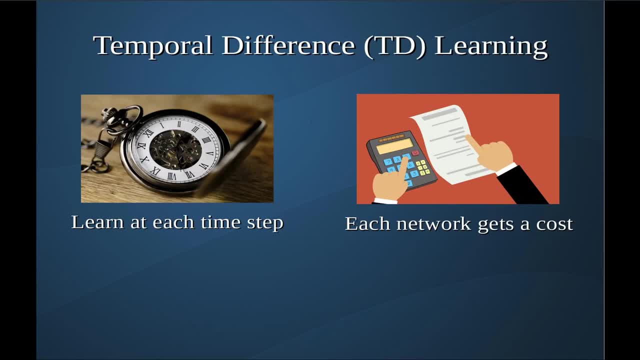 the other for updating our actor To calculate our costs. we want to generate a quantity we'll call delta, and it's just given by the sum of the current reward and the discounted estimate of the new state and then subtracting off the value of the current state. Keep in mind that 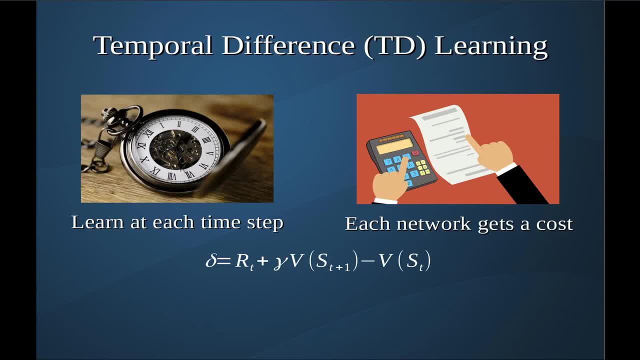 the value of the terminal state is identically zero, so we'll need a way to take this into account. The cost for the critic is going to be delta squared, which is kind of like a typical linear regression problem. The cost for our actor is a little more complex. We're going to multiply. 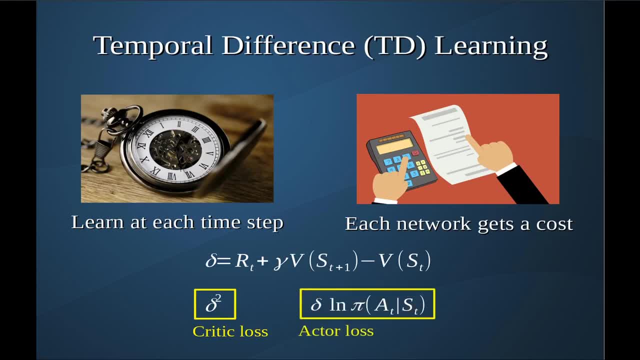 this delta by the log of the policy for the current state and action the agent took. The reason behind this is a little complex and it's something I go into more detail about in my course or you can look for it in the chapter on policy gradient methods in the free textbook by Sutton. 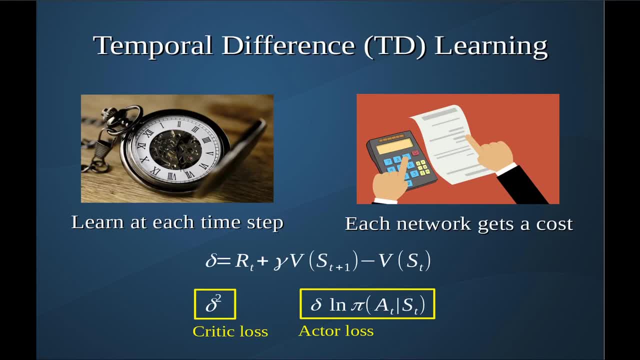 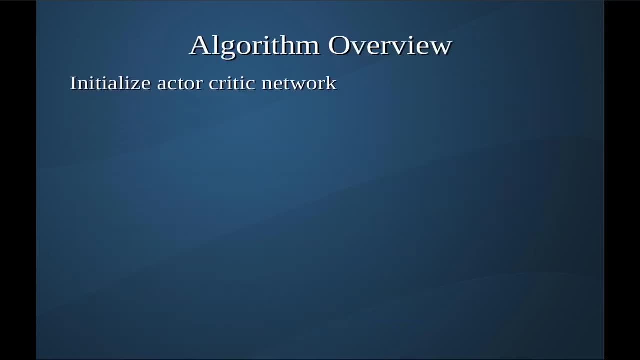 and Bardo. So let's talk implementation details. We're going to implement the following algorithm: Initialize a deep neural network to model the actor and critic. Repeat for a large number of episodes. Reset the score. terminal flag and environment. While the state is not terminal, select an action based on the current state of the environment. 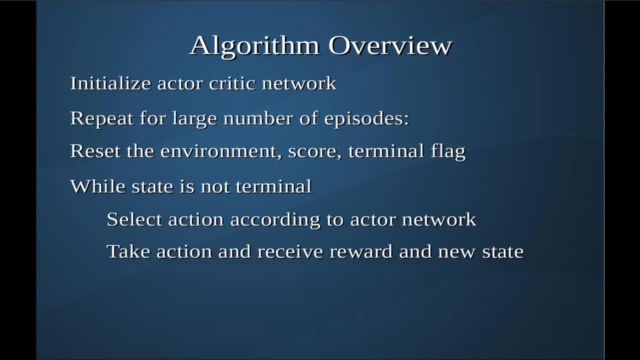 Take the action and receive the new state reward and terminal flag from the environment. Calculate delta and use it to update the actor and critic networks. Set the current state to the new state and increment the episode reward by the score. After all the episodes are finished. plot the trend in scores to look for evidence of learning. 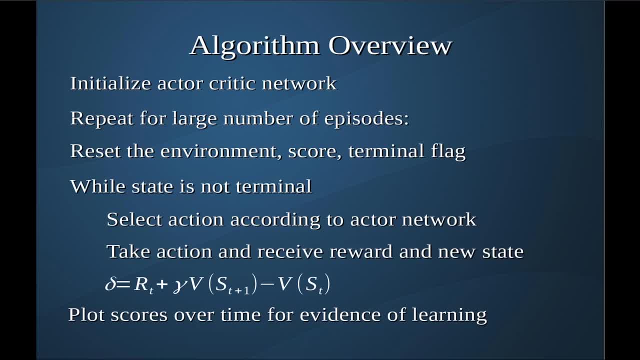 This should be an overall increase in the score. You will see lots of oscillations because actor-critic methods aren't really stable, but the overall trend should be upward. Another thing you may see is that the score can go upward for a while and then fall off a cliff. This isn't uncommon because actor-critic methods are quite 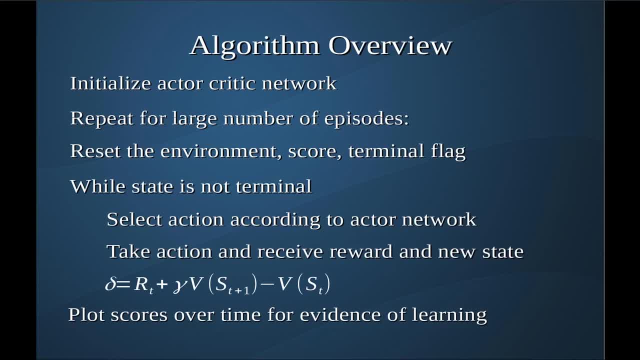 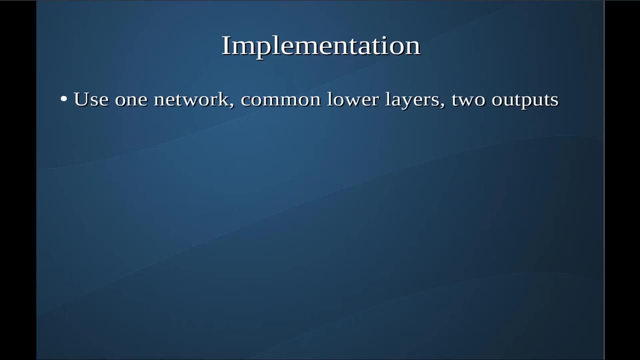 brittle and they're really not the best solution for all cases, but they are a stepping stone to more advanced algorithms. Other important implementation details: You can use a single network for both the actor and critic, So you have common input layers and two outputs, one for the actor and one for the critic. This has the benefit that we don't have. 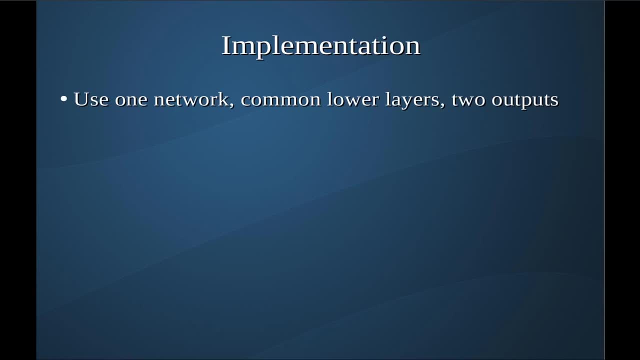 to train two different networks to understand the environment. You can definitely use an independent actor and critic. it just makes the learning more difficult for an algorithm that is already pretty finicky. We'll let it play almost 2000 games with a relatively large deep neural network. 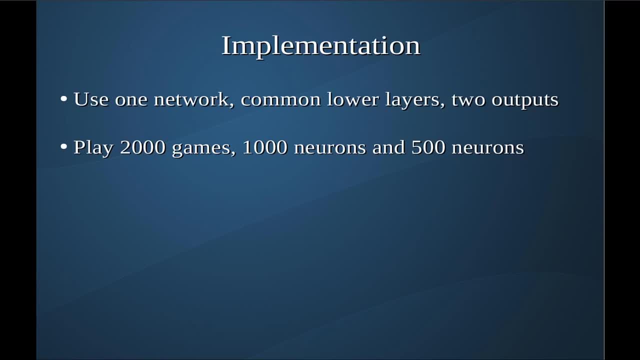 something like about 1000 units in the first hidden layer and 500 units in the second. The hard part is going to be the actor. As I said earlier, the actor models the policy, which is a probability distribution. The actor layer will have as many outputs as our actions and we use a. 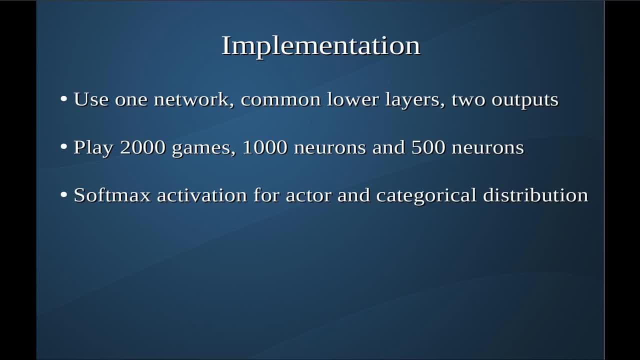 softmax activation, because we're modeling probabilities and they had better sum to one. When selecting actions. we're going to be dealing with discrete action spaces, So this is what is called a categorical distribution. We're going to want to use the tensorflow underscore probability. 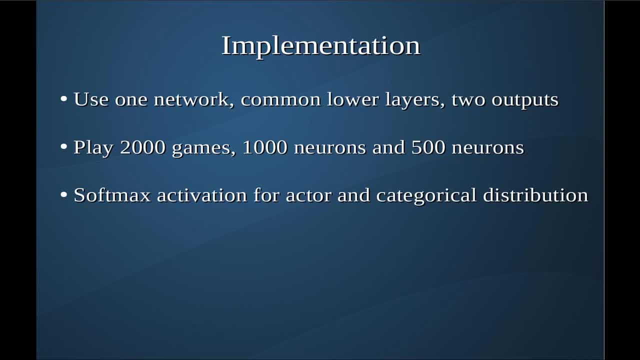 package for the categorical distribution and then use the probabilities generated by the actor layer to get this distribution, which we can then sample and use the built in log function for our cost function. As far as the structure of our code, we're going to have a class for our actor critic network and that will live in its own file. 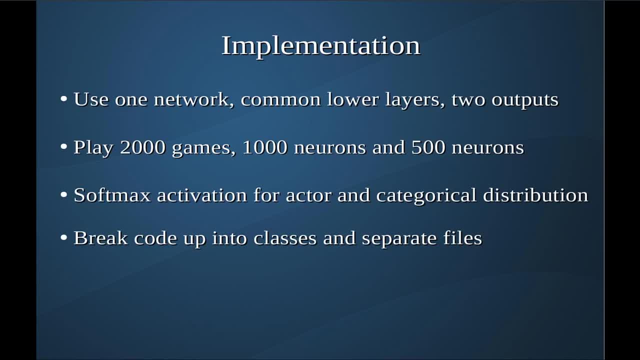 We'll also have a class for our agent and that will have the functionality to choose actions, save models and learn from its experience. That goes in a separate file. The main loop is pretty straightforward, but it does go in its own file as well. 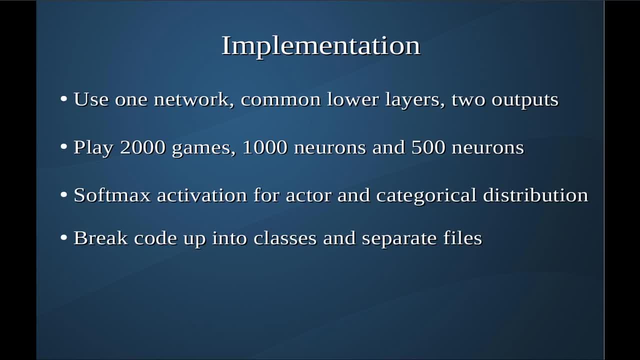 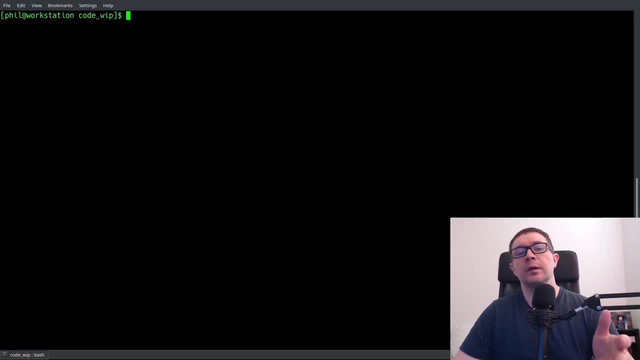 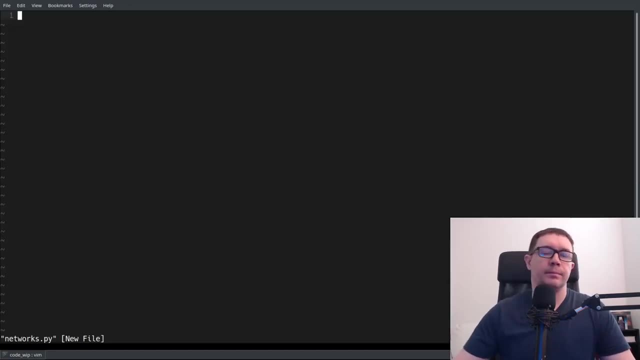 Okay, now that we have all the details out of the way, let's go ahead and get started coding this. So, now that we have all of our lectures out of the way, we're going to go ahead and proceed with the coding. We're going to start with the networks. We begin, as always, with our imports, So we will. 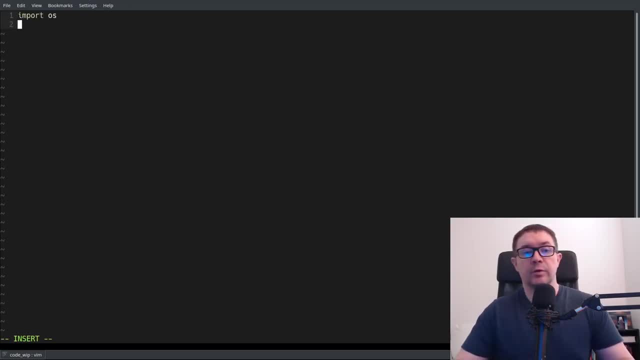 need os to handle file joining operations for model checkpointing. We will need keras And we will need our layers, which for this example, it's just going to be a dense layer. so we will have our actor critic network and you see a case of converging engineering here where tensorflow and pytorch both have you. 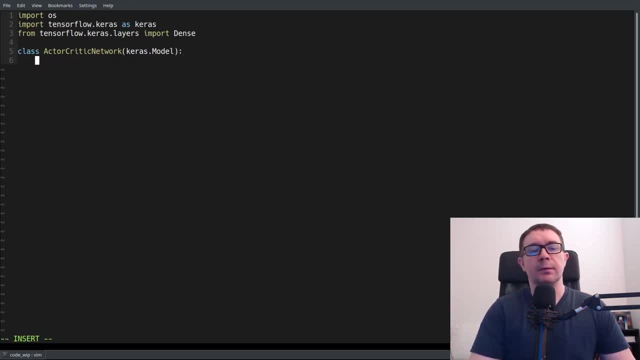 derive your model class from the base model class and we can go ahead and define our constructor that will take a number of actions. as input, the number of dimensions. for the first fully connected layer, we will default that to 1024, and for the second, we will default it to 512. 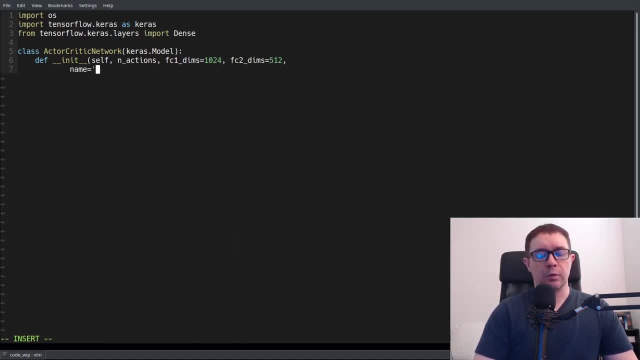 we will have a name for model checkpointing purposes and a checkpoint directory- very important. you must remember to do a make directory on this temp slash actor critic before you attempt to save a model, otherwise you're going to get an error. the first thing you want to do is call your super constructor. 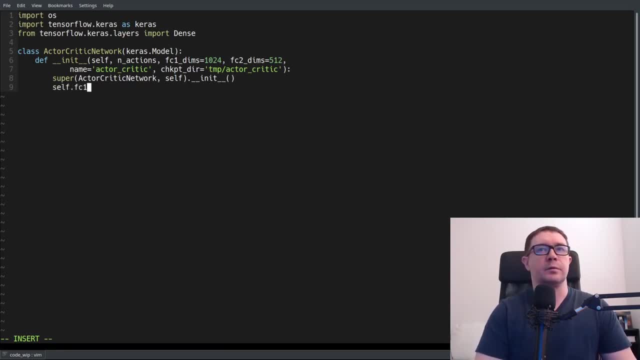 and then go ahead and start saving your parameters now. also very important for our class that we've derived from the base class, in this case the actor critic network class. we have to use model name instead of name, because name is reserved by the base class. so just be aware of that. not a huge deal. 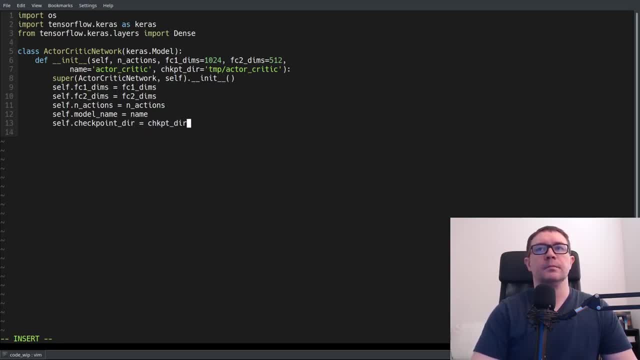 checkpoint directory and then we'll have our file and that will be os path. join the directory name plus underscore ac. i like to use underscore algorithm, in this case ac for actor critic, in case you have one directory that you use for many different algorithms. if you're just using, like say, a working directory, you don't want to confuse the model types otherwise. 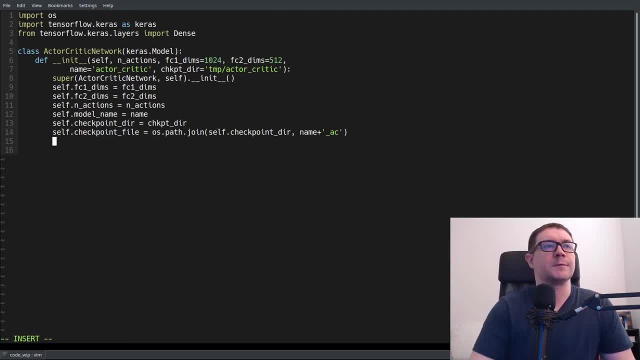 if you have a good model saved, you don't want to override it with something else. now we'll go ahead and define our layers and that will be the fully connected dense layers. the neat thing about keros is that the number of input dimensions are inferred, so we don't have to specify it. that's why we don't have an input dims. 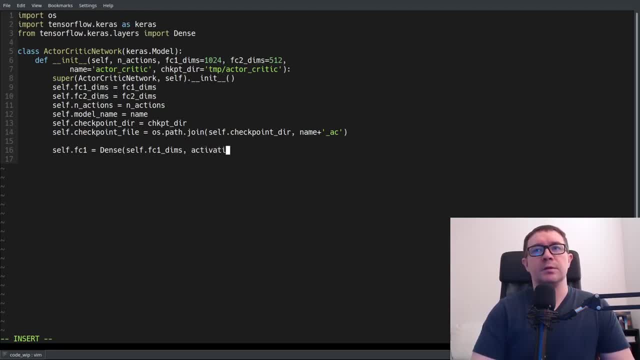 for our constructor and it will output fc1 dims with an activation of value. fc2 will be similar and then we will have two separate outputs. so we have two common layers and then two independent outputs: one for the value function, and that is single valued with no activation, and the second is our policy pi and that will output an actions with a soft max. 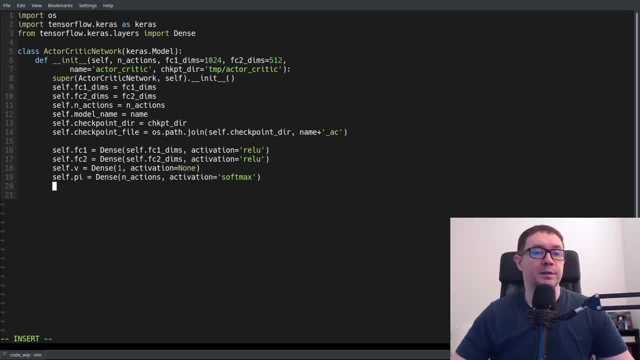 activation. recall that the policy is just a probability distribution, so it assigns a probability to each action and those probabilities have to add up to one because the policy is a probability. That's kind of what probabilities do, right? Next we have to define our call function. 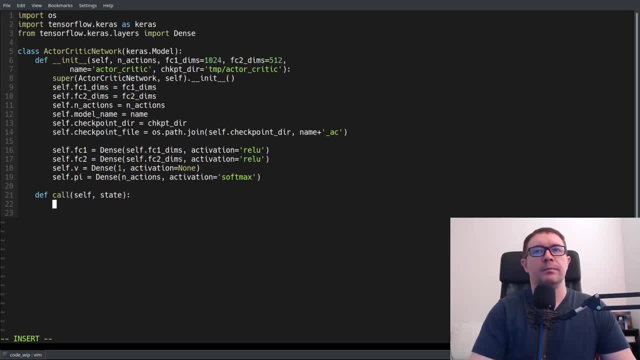 This is really the feed forward- If you're familiar with that- from PyTorch. So we'll just use some generic name like value- It doesn't really matter- And pass it to the second fully connected layer And then get our value function and our policy pi. 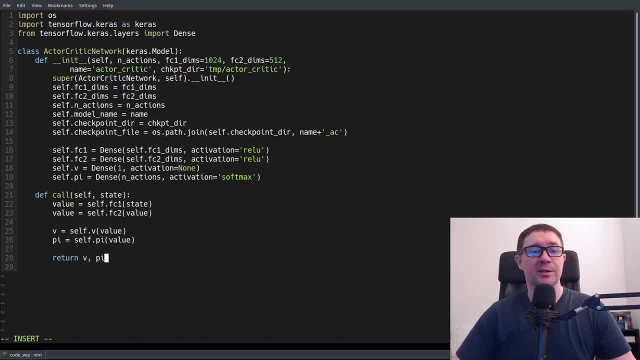 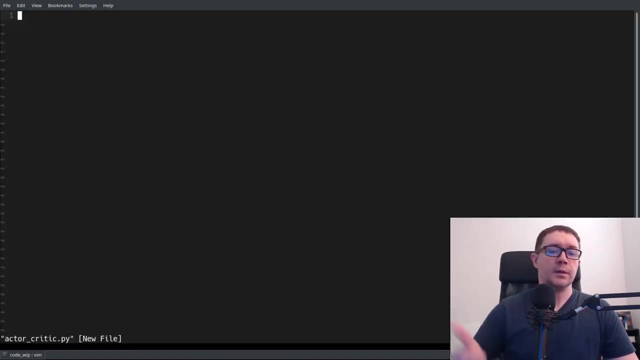 And then return both the value function and the policy pi. So that is really it for the actor critic network. All of the interesting functionality happens in the agent class, So let's go ahead and start writing the agent class. So we begin, as always, with our imports. 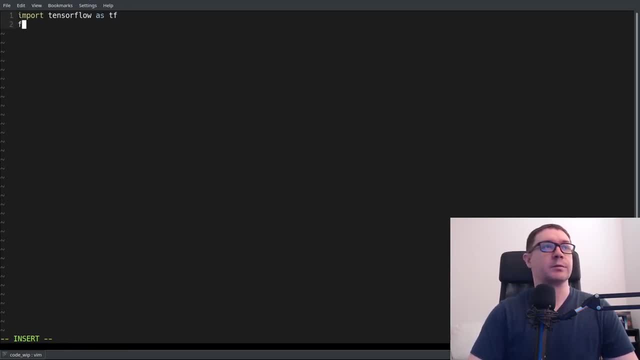 We will need tensorflow, We will need our optimizers. In this case, we're going to use the tensorflow. In this case, we're going to use an atom optimizer Probability. We will need tensorflow probability to handle our categorical distribution, to model our policy directly. 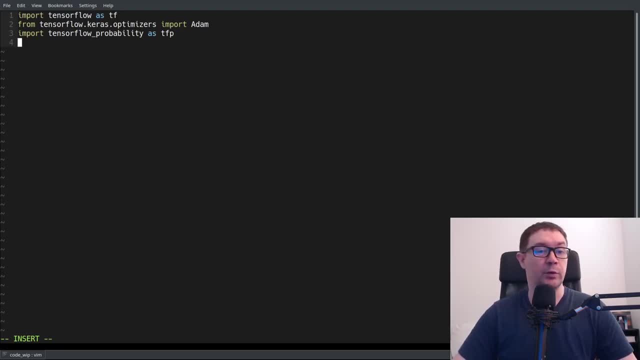 You have to do a pip install tensorflow probability before you can run this. This is a separate package from tensorflow And we will also need our actor critic network, So let's go ahead and code up our agent. So our initializer is pretty straightforward. 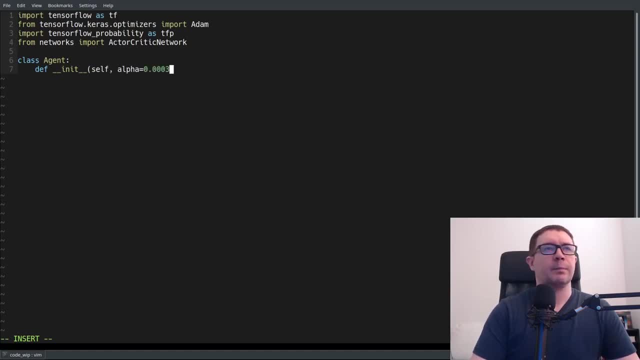 We will need some default learning rate. I'm going to use 0003.. It doesn't really matter. I'm going to pass in a specific learning rate in the main file. We will have a gamma of 0.99 and default inactions of some number, like say 2.. 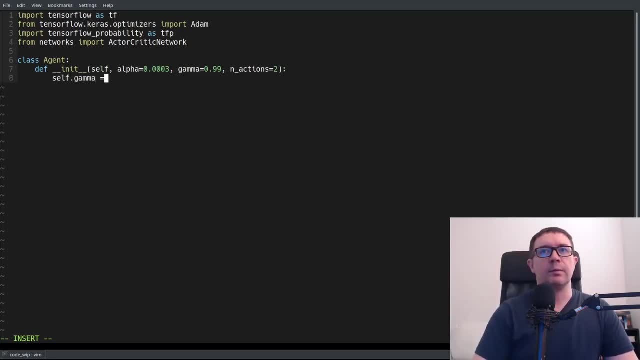 So we're going to go ahead and save our parameters. We'll call the gamma as our discount factor. We're going to need a variable to keep track of the last action we took. This will be a little bit more clear when we get to the learn function. 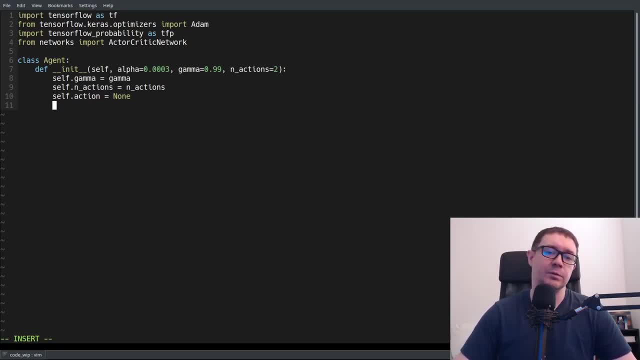 It has to do with the way we calculate the loss, because we have to use a gradient tape for tensorflow2.. It's just a bit of a workaround for how tensorflow2 does things. We need our action space for random Another action selection. That's just a list of actions from 0 to an actions minus 1.. 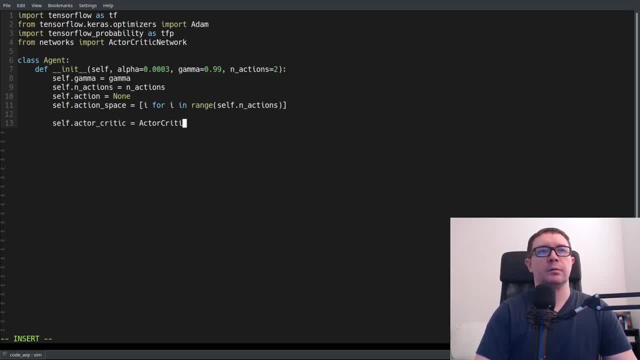 We need our actor critic. We want to make sure to specify the number of actions And we want to compile that model. So actor critic compile with an atom optimizer and learning rate Defined by alpha. Next we have the most basic functionality of our agent. 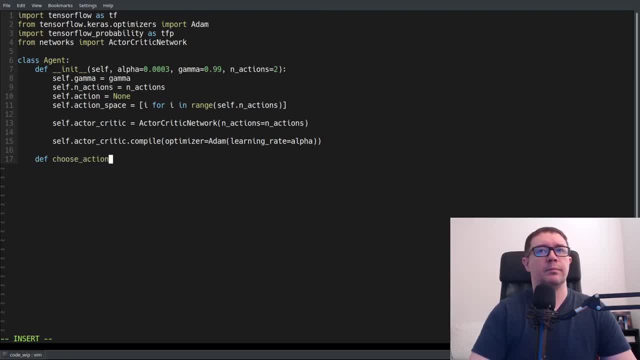 the functionality to choose an action, And that takes the current state of the environment as input, which we have to convert to a tensor. And, in particular, we have to add an extra dimension, a batch dimension, The reason being that the deep neural network. 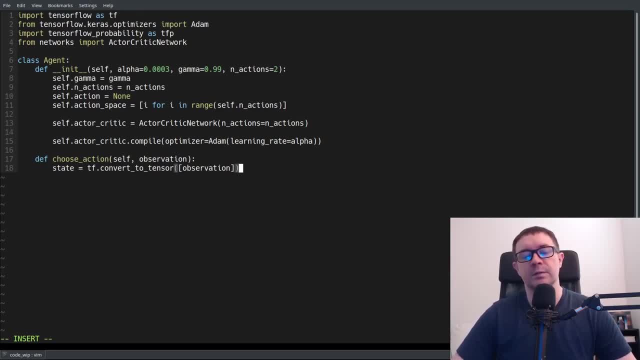 it expects a batch of inputs, And so you have to have something other than a 1D array. It has to be two-dimensional, So we just add an extra dimension along the zeroth dimension, So then we will feed that through our deep neural network. 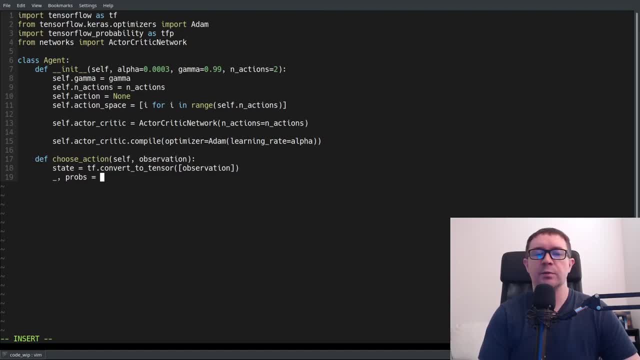 We don't care about the value of the state for the purpose of choosing that action, So we just use a blank And we will get the probabilities by passing the state through the actor critic network And then we can use that output, the probabilities defined by our neural network. 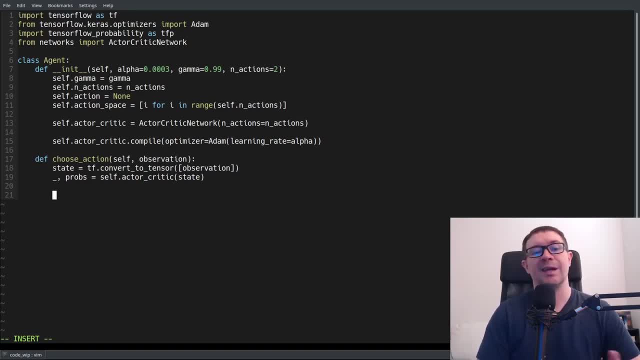 to feed into the actual tensor flow probabilities, categorical distribution, and then use that to select an action by sampling that distribution and getting a log probability of selecting that sample. Sorry, that's TFP, Categorical and probabilities given by probs And our actual action will be a sample of that distribution. 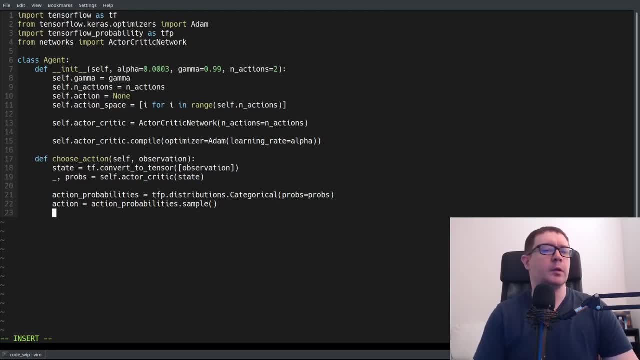 And we don't actually need the log prob at this stage. We will need the log problem when we calculate the loss function for our deep neural network, but we don't need it now And it doesn't make sense, or rather it doesn't actually work- to save it to a list. 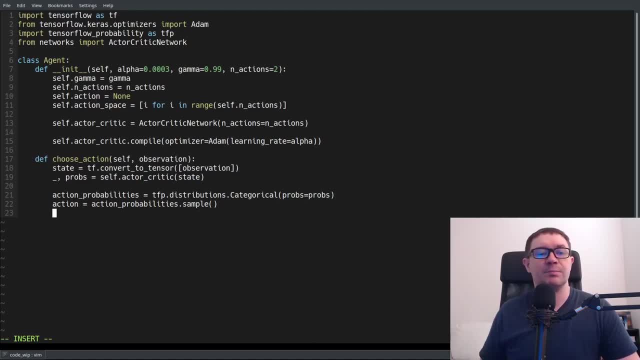 let's say for use later here, because this calculation takes place outside of the gradient tape. Okay, TensorFlow 2 has this construct of the gradient tape. It's pretty cool. It allows you to calculate gradients manually, which is really what we want to do here. 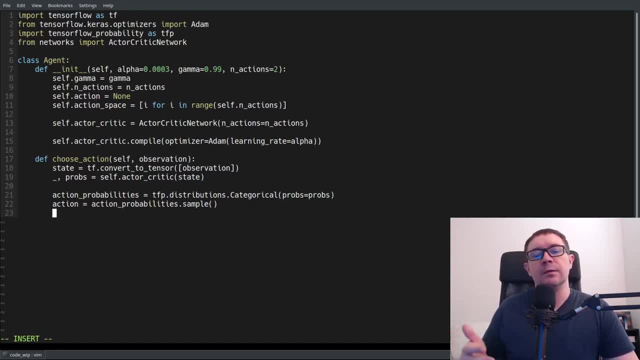 But anything outside of that tape doesn't get added to the calculation for back propagation, So the log prob doesn't matter at this point, So why bother calculating it? One thing we do need, however, is the action that we selected, So we will save that in the action variable. 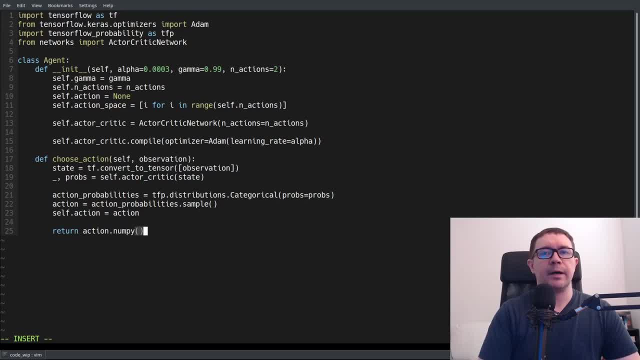 and we will return a NumPy version of our action, because action is a TensorFlow tensor which is incompatible with the OpenAI GIMP. It does, however, take NumPy arrays And we want the zeroth element of that because we added in a batch dimension. 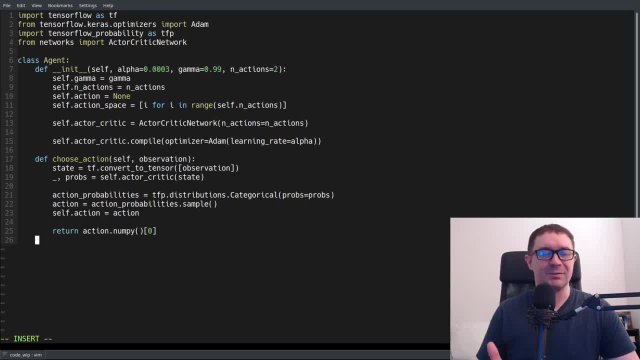 for compatibility with our deep neural network And a little bit confusing, but that is what we have to deal with. Next let's do a couple of bookkeeping functions to save and load models. Those will take any inputs And so it will save the weights of the network. 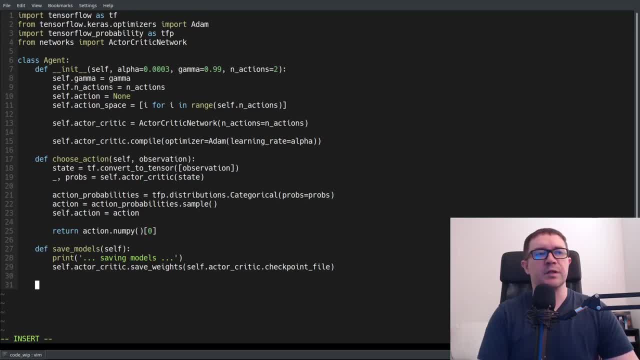 to the checkpoint file. We do the inverse operation to load models And we will load weights from a checkpoint file. So that is it for the basic bookkeeping operations. Next we have the real heart of the problem: the functionality to learn. 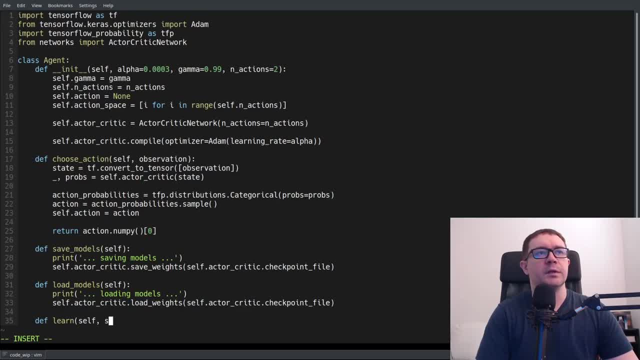 So this will take a number of inputs. We'll take the state reward received, new state and terminal flag as input. The first thing we want to do is convert each of those to TensorFlow tensors and make sure to add a batch dimension. 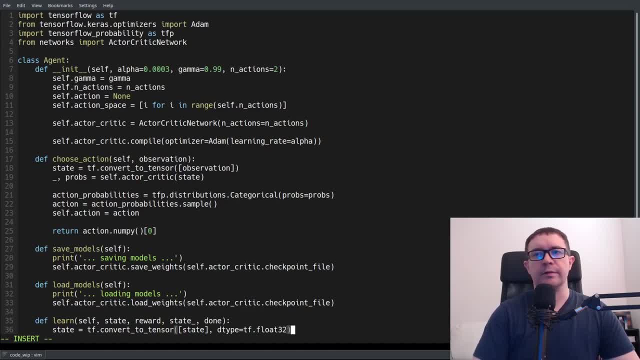 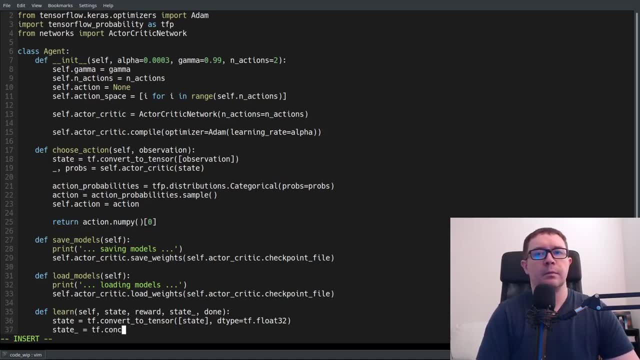 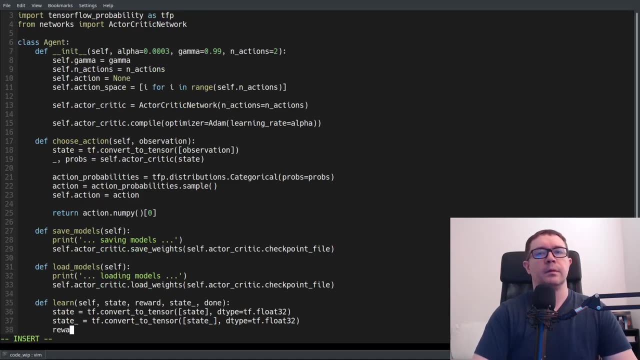 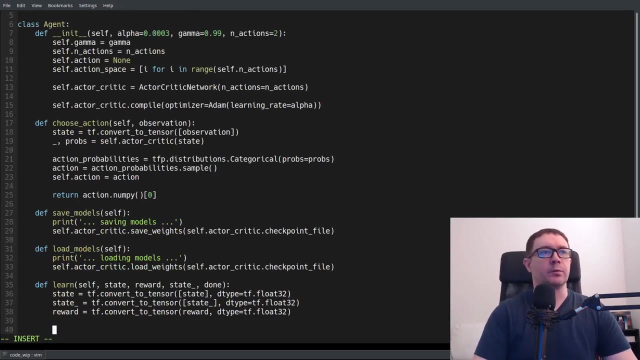 And I like to be really pedantic with my data type, so I will cast it to TF, float 32.. And we don't have to add a batch dimension to the reward, because it is not fed to a deep neural network. So now we get to calculate our actual gradients using something. 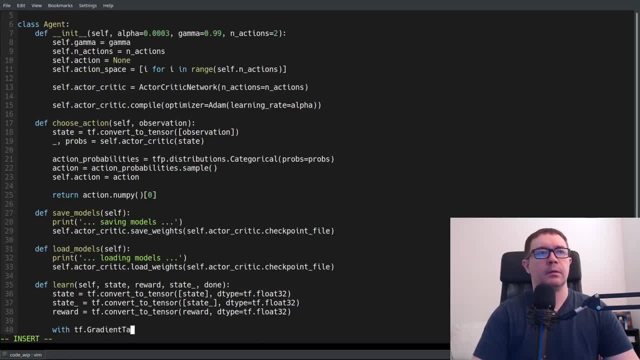 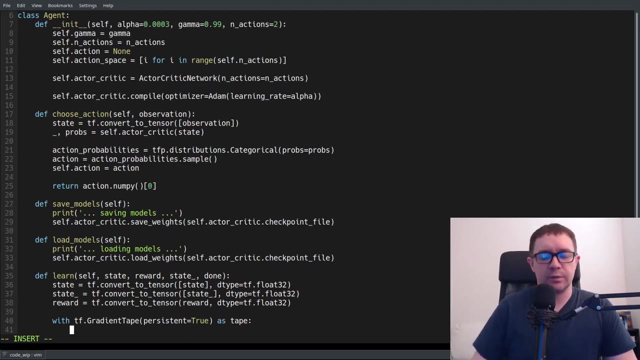 called the gradient tape And we'll set persistent to true, And I'm not actually sure that's needed. I'm going to go ahead and experiment with that when we go ahead and run the code, But I have it that way. I might have just copied and pasted code from somewhere else. 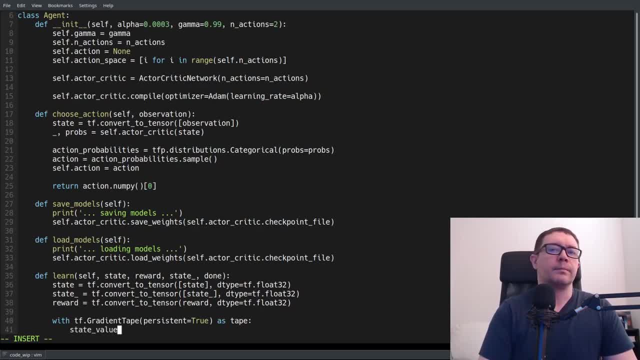 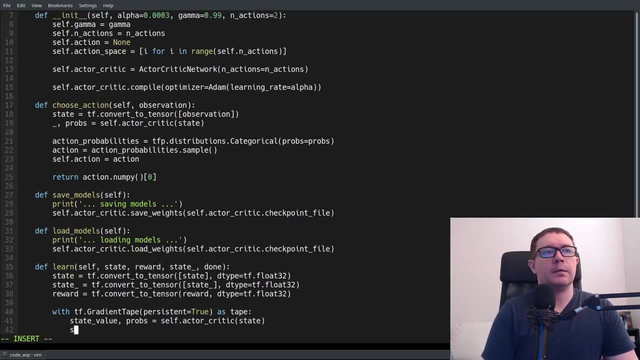 So let me double check. But we want to feed our state, a new state through the actor critic network and get back our quantities of interest. So we feed the current state and then the new state And then we get back our quantities of interest. 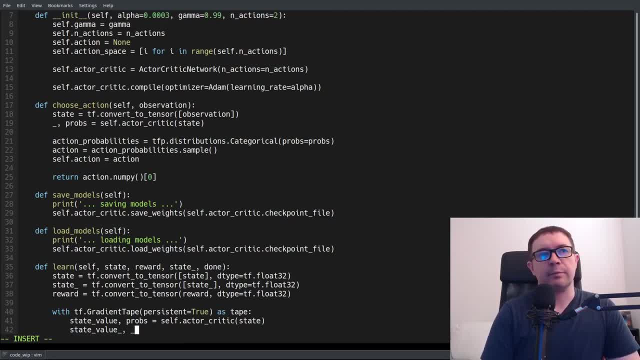 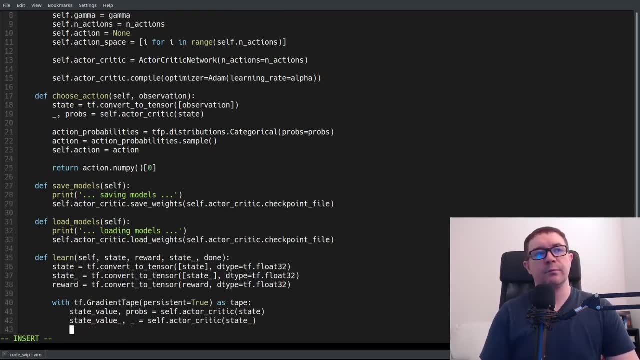 So we feed the current state and then the new state. But for the new state we don't care about the probabilities, We just care about the value. And that is for calculation of our delta. But for the calculation of our loss we have to get rid of that batch dimension. 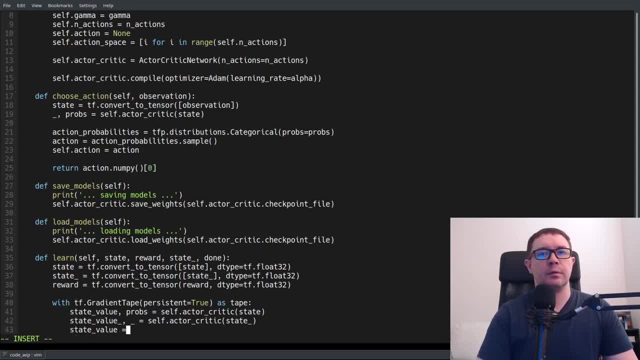 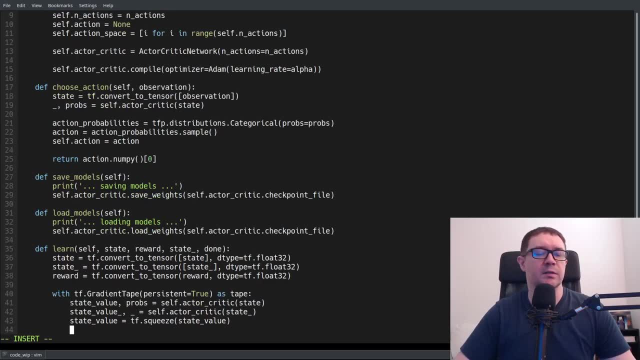 So we have to squeeze these two parameters, And the reason you have to do that is because the loss works best if it's on a one-dimensional quantity. And the reason you have to do that is because the loss works best if it's on a one-dimensional quantity. 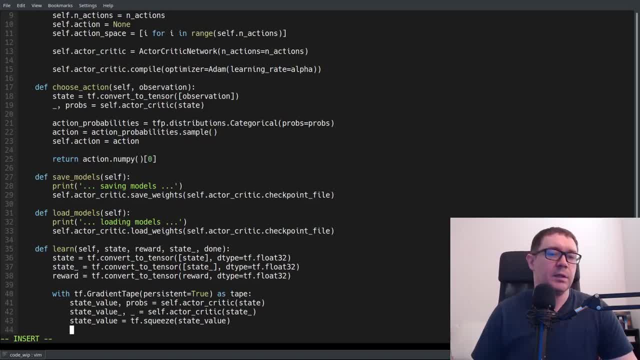 Or rather a scalar value rather than a scalar value inside of brackets. So it has to be a scalar instead of a vector containing a single item O. It's just something we have to do. I encourage you to play around with it, to double check me on that. 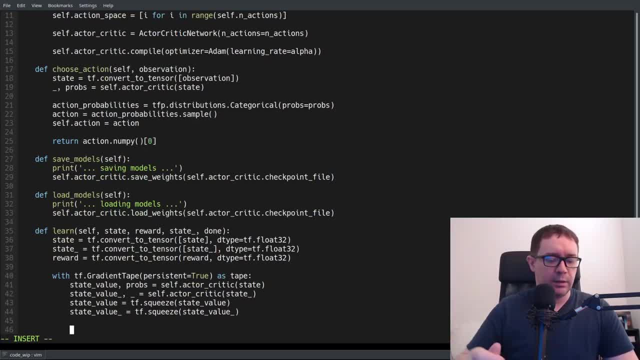 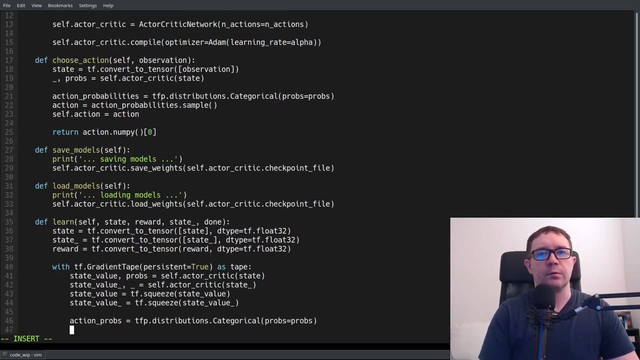 I move between distributions, excuse me, frameworks, So sometimes stuff isn't always 100% necessary, even if it doesn't hurt anything. So we need our action Probabilities for the calculation of the log prob, TFP distributions categorical, And we define our probes by the output of our deep neural network. 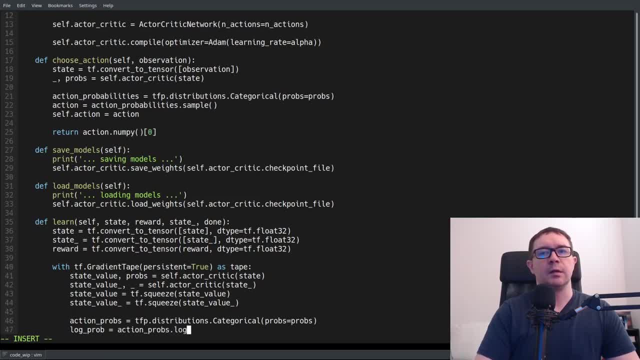 And then our log prob is action probes, dot, log prob of the self dot action And this is the action that we saved up at the top when we calculate the action for the agent. So this is the most recent action. Then we calculate our delta. 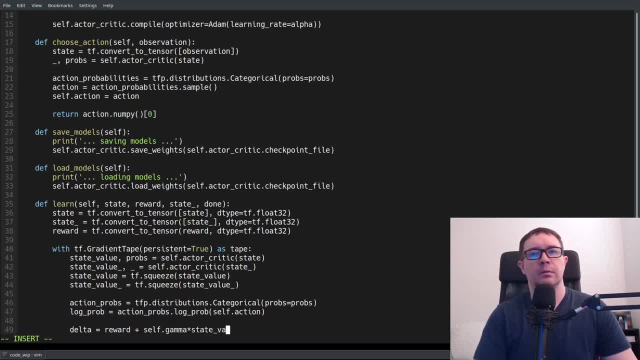 That is a reward plus gamma multiplied by the value of the new state, times 1 minus int of done. And the reason for that is that the value of the terminal state is identically zero, because no returns, no rewards follow the terminal state, So it has no future value. 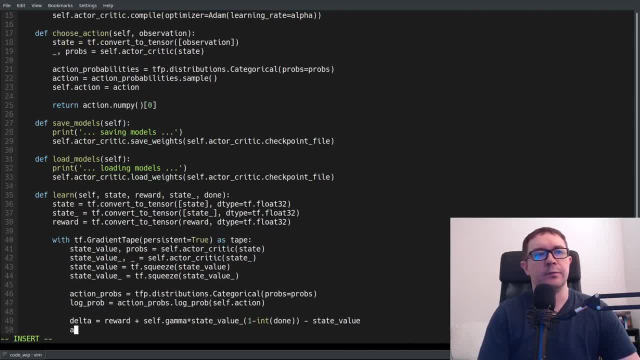 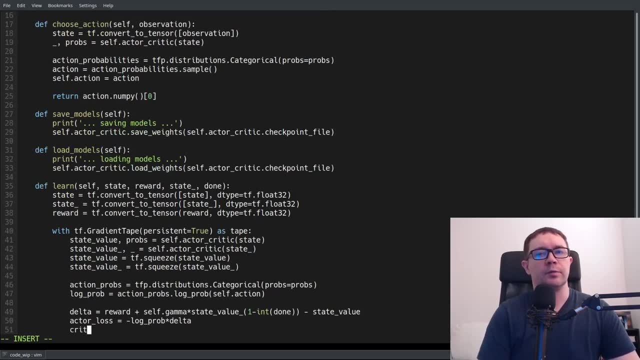 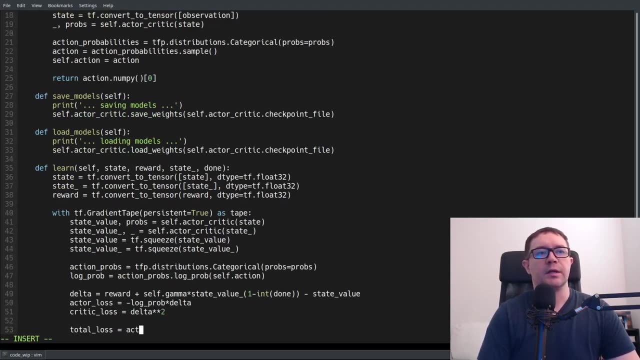 And I subtract off the state value. So our actor loss is minus log prob times that delta And we do the equation times that delta and the critic loss is delta squared and the total loss equals after loss plus critic loss, And then we can go ahead and calculate our gradients. 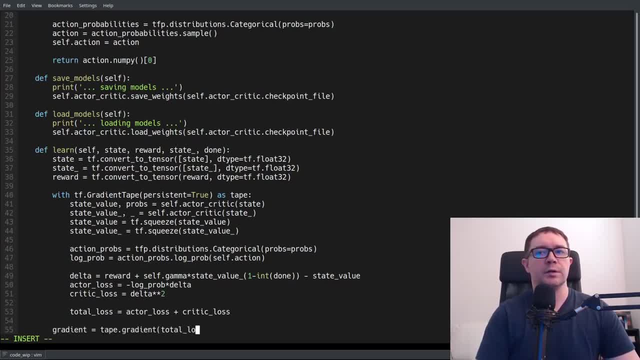 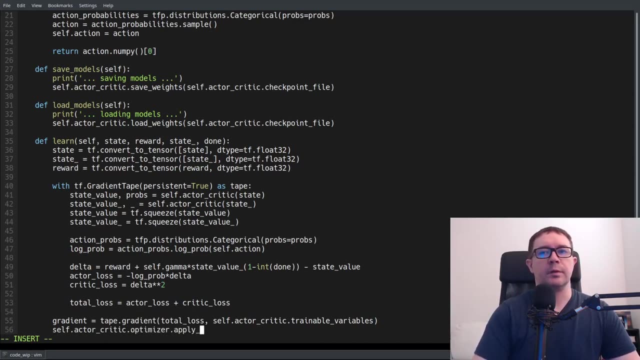 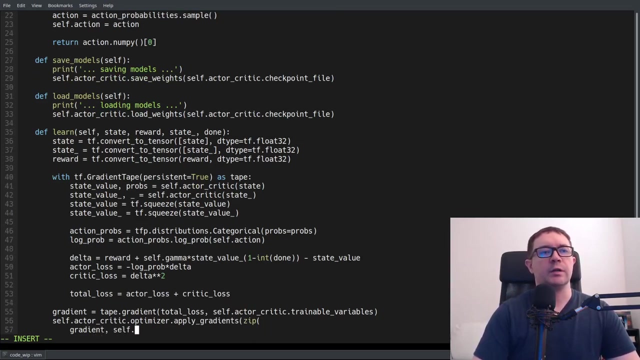 So our gradient is tapegradient- total loss with respect to the trainable variables- And this expects a zip as input. So we're going to zip the gradient and the trainable variables. All right, And that is it for the actor critic functionality. So I'm going to come back to this. 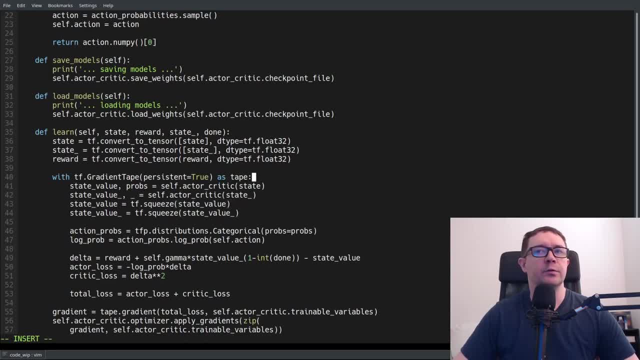 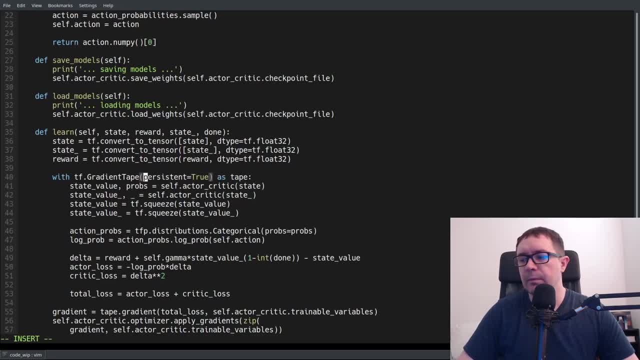 I need this in the case when we have- if we were to have, say, separate actor and critic networks and had to calculate gradients with respect to two separate sets of trainable variables. I believe that's when the persistent equals true would be necessary. 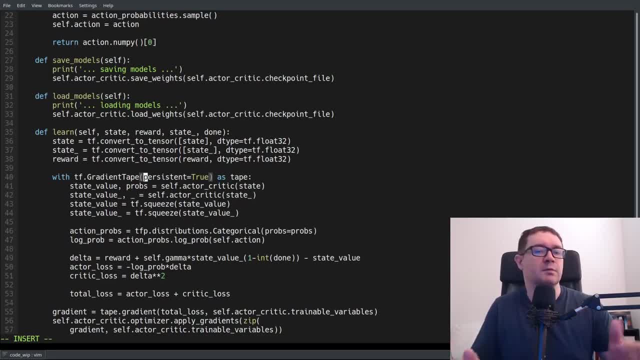 And when we had coupling between the loss of one network and the other. it's so that it keeps track of the gradients after it does the back propagation, kind of like in PyTorch, where it throws it away and you have to tell it to retain the graph. 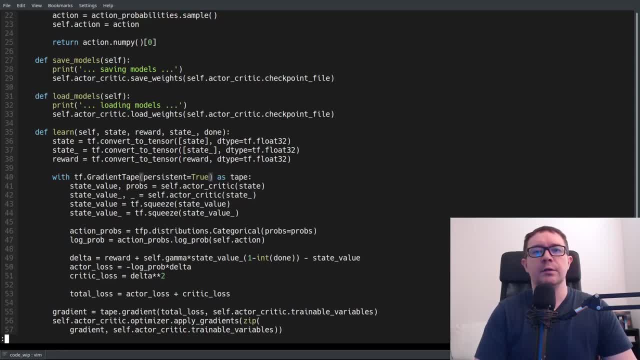 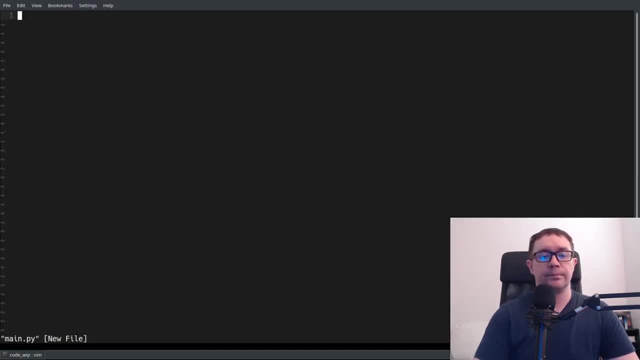 I'll double check on that, though. So let's go ahead and write and quit, and then we're ready to go ahead and code up our main file. So, with our imports, we will need Jim, We will need NumPy, We will need our agent. 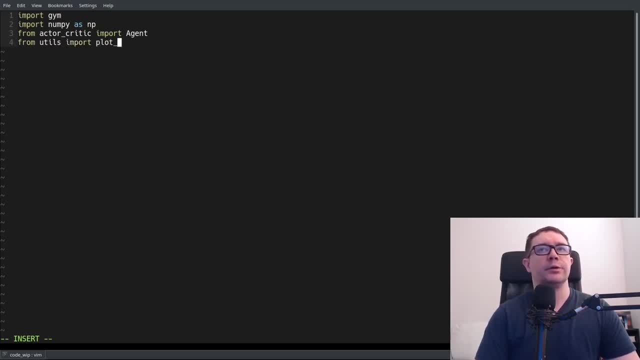 We will need our plot learning curve function. I'm not going to go into any detail. All this is just a function to plot data using plot live, with some labeled axes. It's nothing really worth going into. First thing we'll do is make our environment. 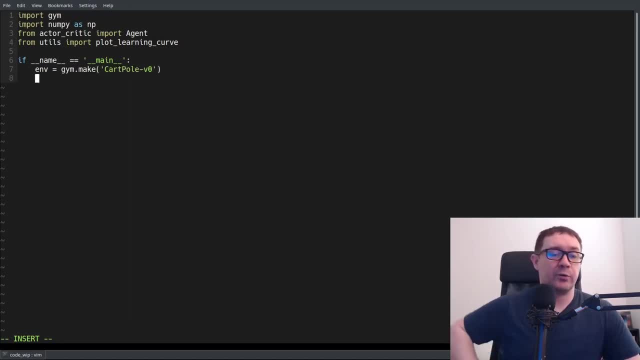 And I'm using the cart pull because it runs very quickly and the actor critic method is quite brittle, quite finicky, You will observe, in many cases where it will achieve a pretty decent score and then a fall off a cliff because the learning rate was just a little bit too high. 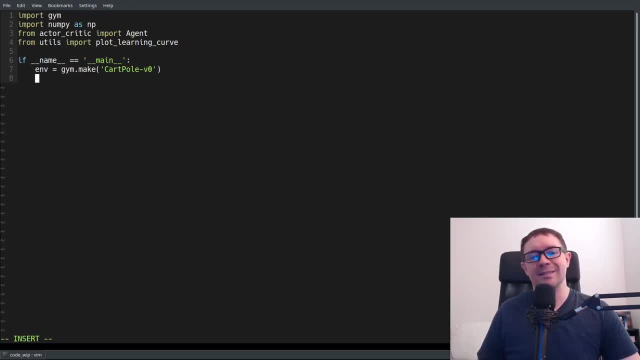 So there are a number of problems with the algorithm and it's easiest to test in a very simple environment. In my course we use the lunar lander environment and I did more hyperparameter tuning to get it to actually get pretty close to beating the environment. 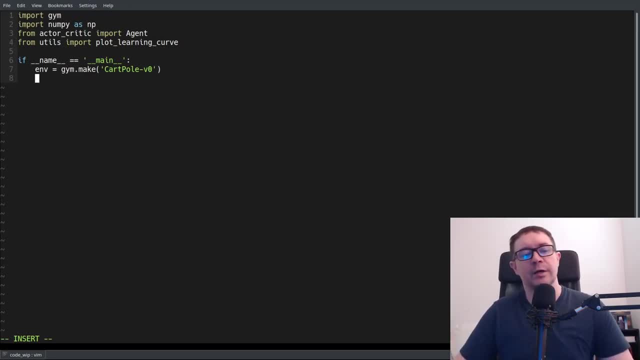 I believe In this case we won't quite beat it. We achieve a high score of like 140 points or so when beating it is 200. But I leave the exercise of hyperparameter tuning to you, the viewer. I got to leave something. 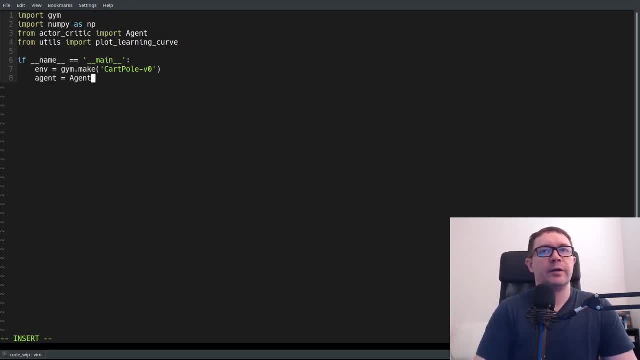 I got to leave something for you to do as well, right, So we'll define our agent with a learning rate of one by 10 to the minus five and a number of actions defined by our environment, action space underscore, And then we'll have, say, 1800 games about 2000 with a file name of cart pull dot PNG. 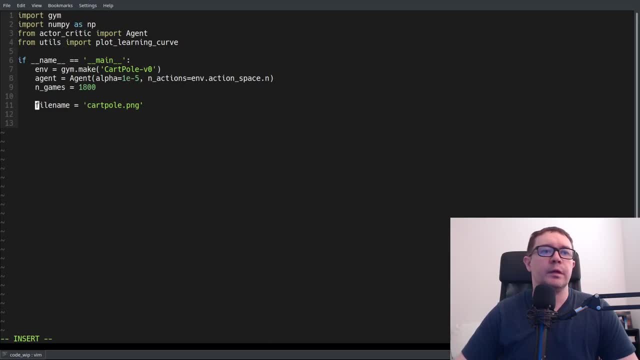 I would encourage you, if you do hyperparameter testing, to put the string representations of those hyperparameters here in the file name, So that way when you look at it later you don't get confused and you know what hyperparameters were used to generate which plot. 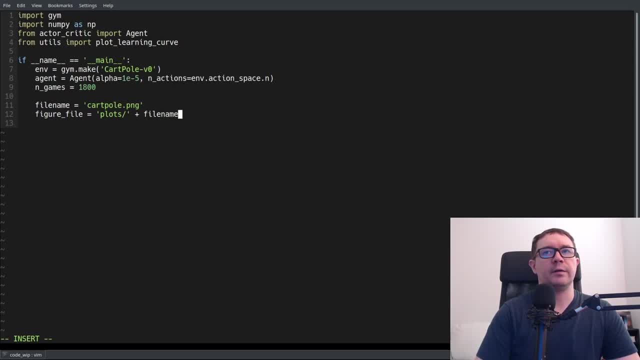 So our figure file is just plots plus the file name. I split it up. You don't have to do it that way. We want to keep track of the best score received and it'll default to the lowest range. So that way the first score you get is better than the lowest of the ranges. 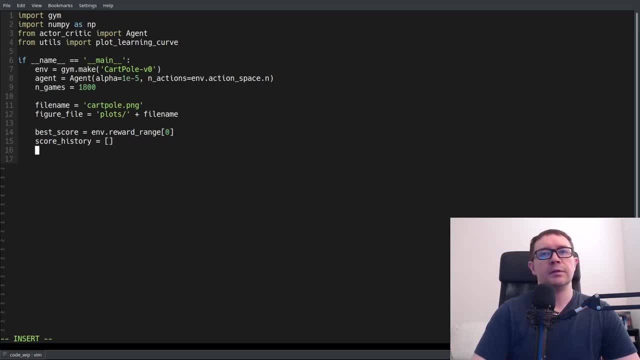 Save your models right away. An empty list to keep track of the score history, A Boolean for whether or not we want to load a checkpoint. So if we're going to load a checkpoint, then we're going to load models, And then, finally, we want to go ahead and start playing our games. 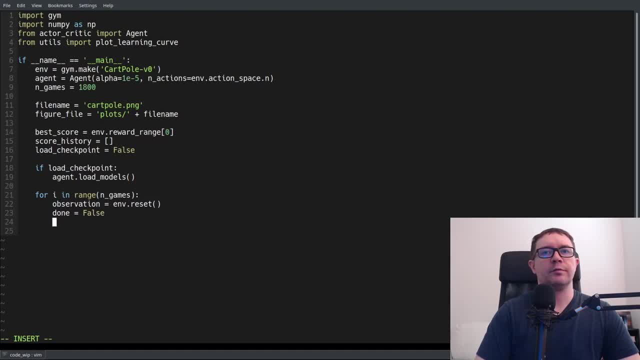 We want to reset our environment, Reset our terminal flag, Set our score to zero And while we're not done with the episode, we can choose an action: Get the new state reward done in info from the environment, Increment our score. If we're not loading a checkpoint, then we want to learn. 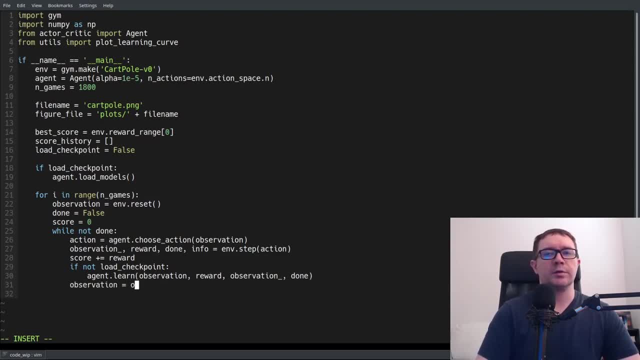 Either way, we want to set the current state to the new state. otherwise you will be constantly choosing an action based on the initial state of the environment, which obviously will not work. You also want to append the score to the score history for plotting purposes and calculate. 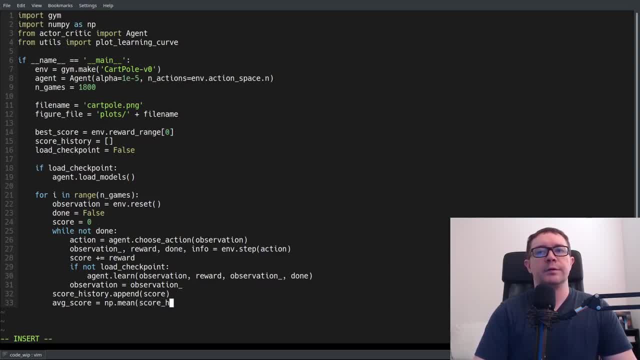 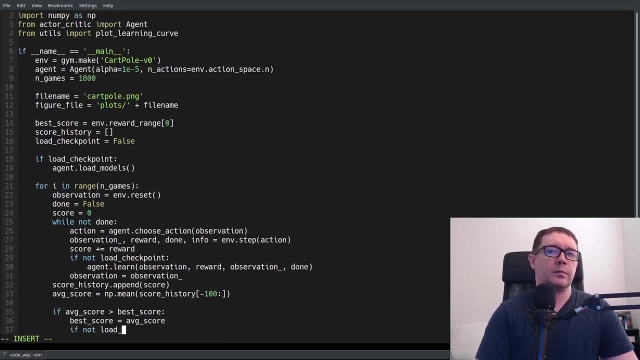 a score, an average score of the previous- I don't know, say 100 games, And if that average score is better than your best score, then set the best score to the average score. And if we're not loading a checkpoint, then save your models. 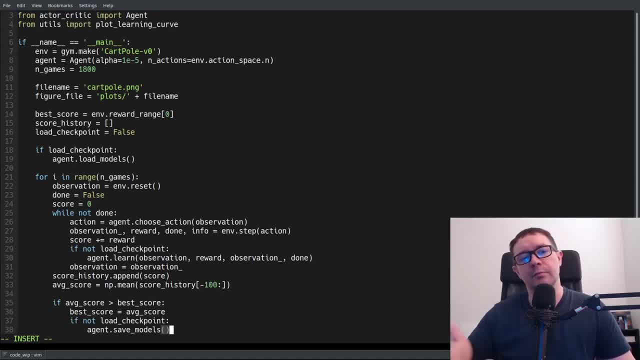 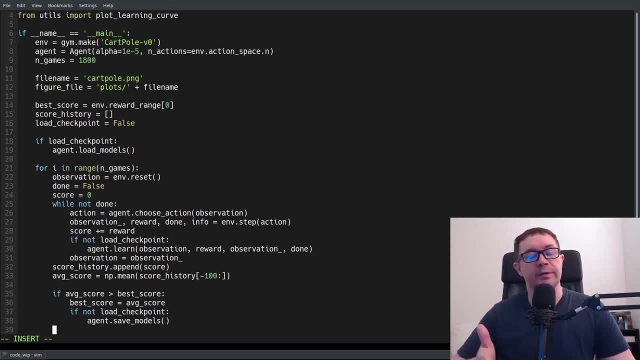 So this inner conditional statement keeps you from overriding your models that had your best scores when you're actually testing. If you just save the model every time, then you'd be overriding your best model with whatever, which may not be the best model. So at the end, if we're not loading a checkpoint, actually we can just plot either way. 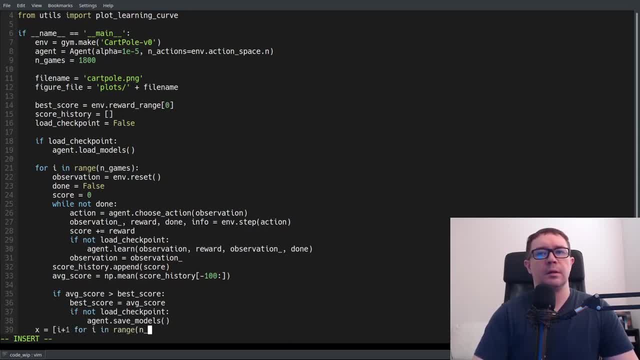 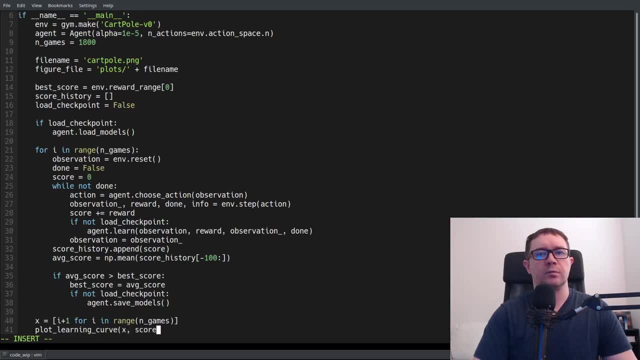 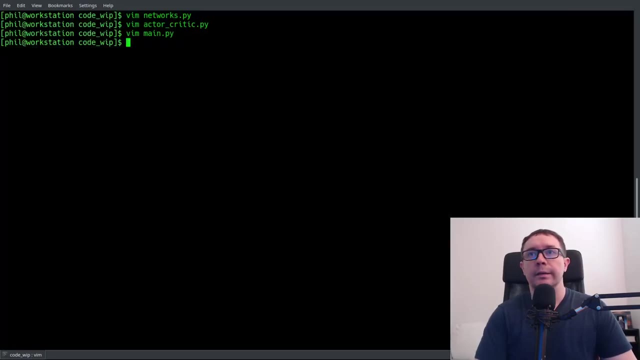 Let's do that. Let's go to our x-axis And plot learning curve, x score Figure file. Okay, Now I have to do a mkdir on plots temp. did I call it temp slash, actor critic? otherwise this stuff won't work. 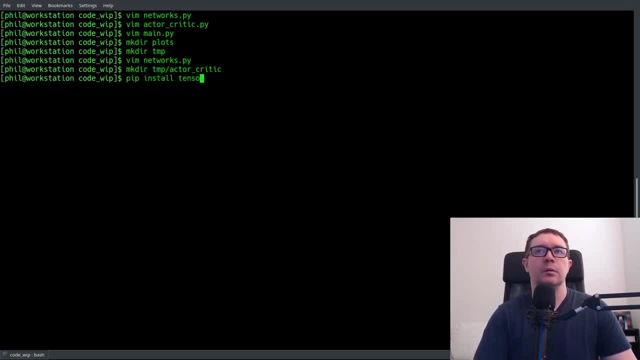 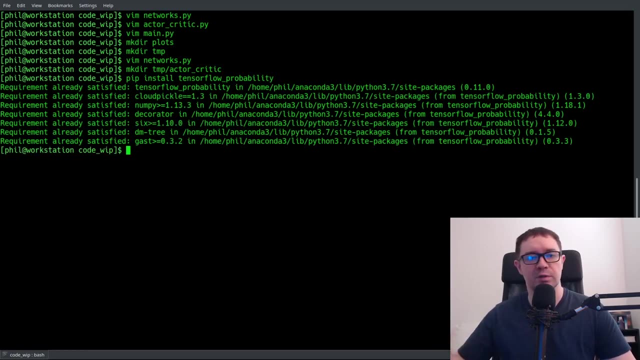 And you also want to do a pip, install flow tensorflow properties. I'm not going to do that, I'm just going to call it. I'm going to call it tensorflow probability, because that is a separate package. Of course, I already have it. 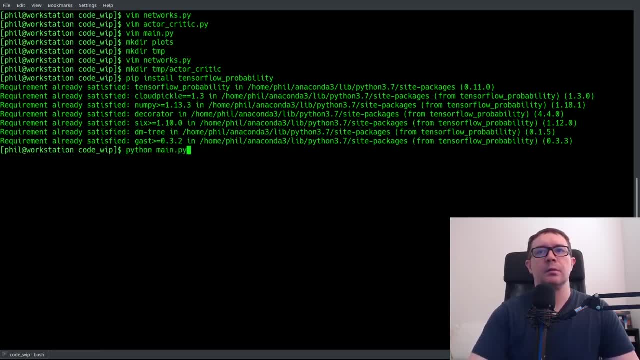 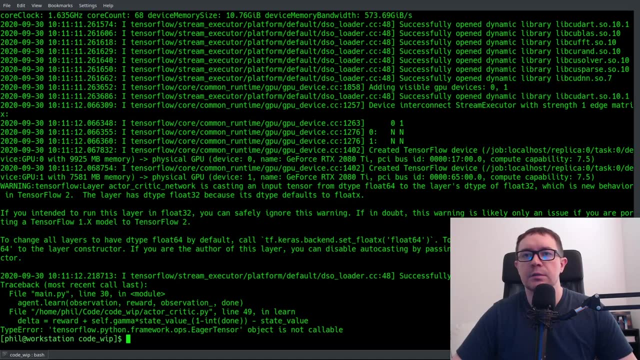 So let's go ahead and try to run this and see if I made any typos. I'm certain, almost certain, I did. So it says something. something is not callable. Oh, that's because I have forgotten my multiplication sign. So that is in line 49.. 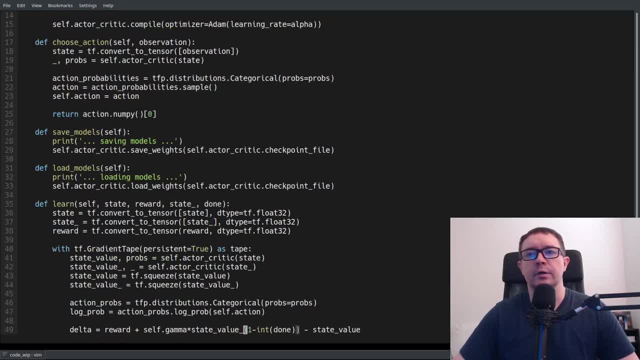 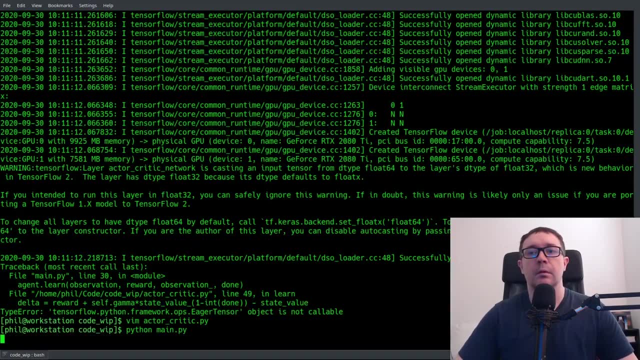 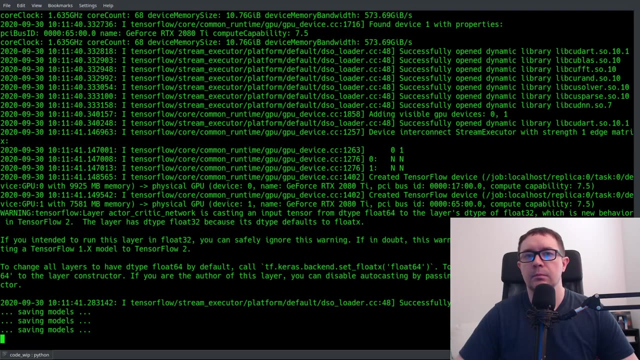 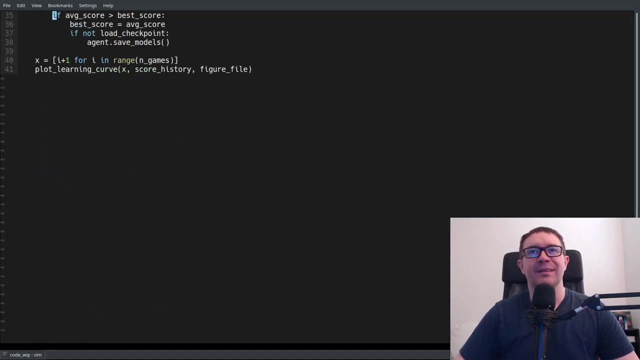 Yeah, Okay, Yeah. It thinks I'm trying to call something here when I really want to multiply. Oh, you know what I did forget? One thing I did forget, of course, is down here. I forgot my debug statement, So let's do this. 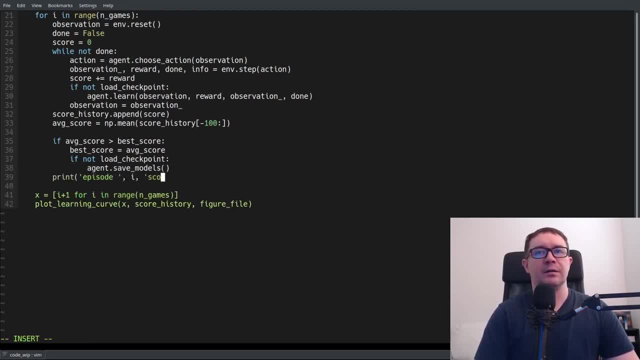 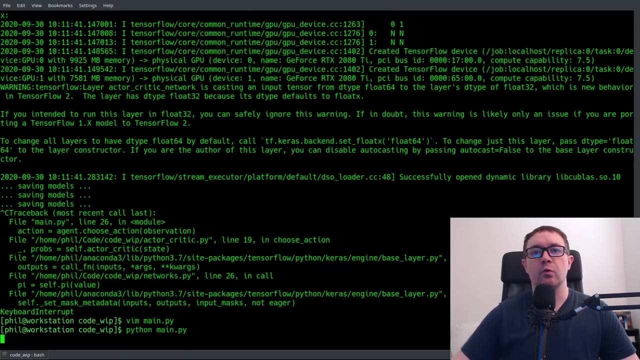 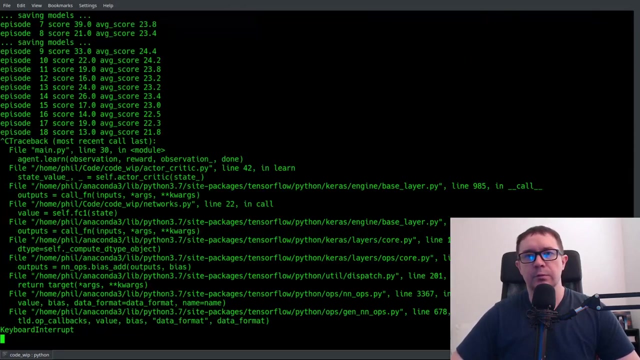 That's pretty funny Episode. I score a percent, one F. Always have to forget something, of course. Okay, there we go. So one other thing I want to do is come back here to actor critic and get rid of this persistent equals true. 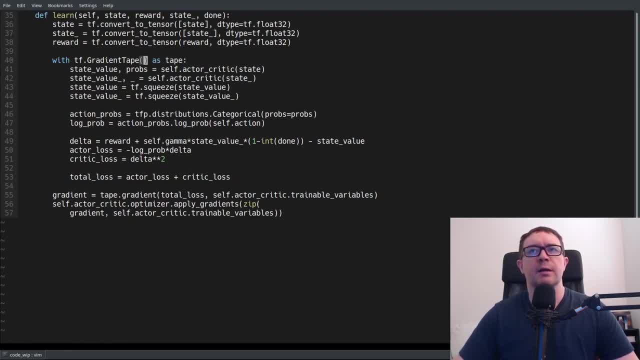 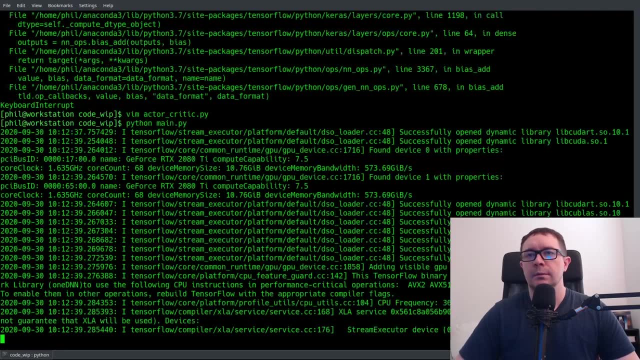 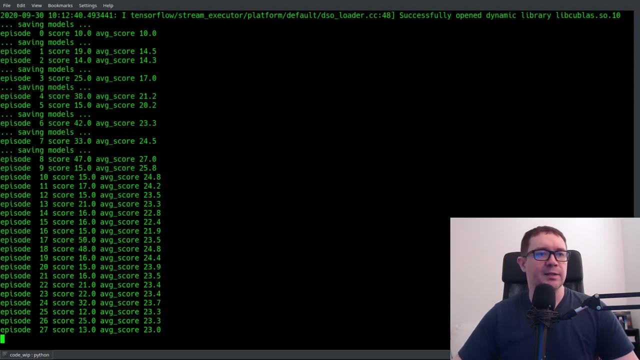 I don't think I actually need this. Sometimes I just copy and paste code and then, as I'm doing the video, I realize: oh hey, I don't always need all that stuff, Okay. so yeah, it does run, Alrighty. so I'm gonna go ahead and switch over to another window where I have let this finish up. 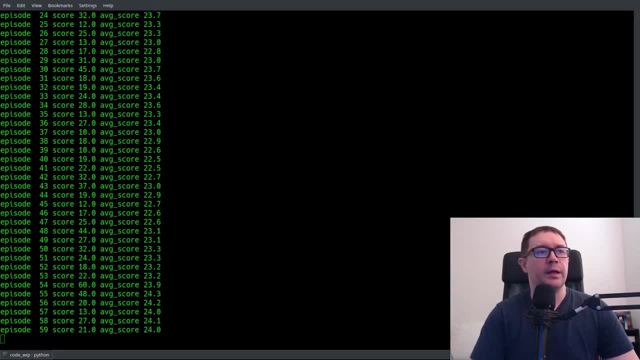 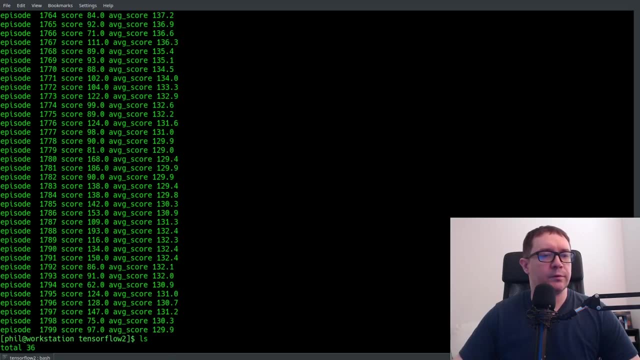 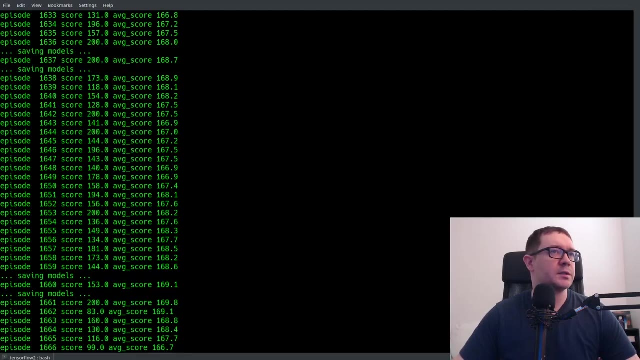 Because there's no point letting it run for another 1800 games. so let's go ahead and check that out. So here you can see the output of the other 1800 games I ran, and it does achieve a score of around a hundred and sixty seven hundred sixty eight, about a hundred seventy points or so. 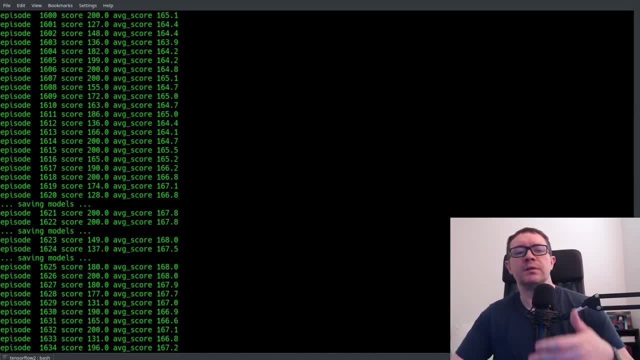 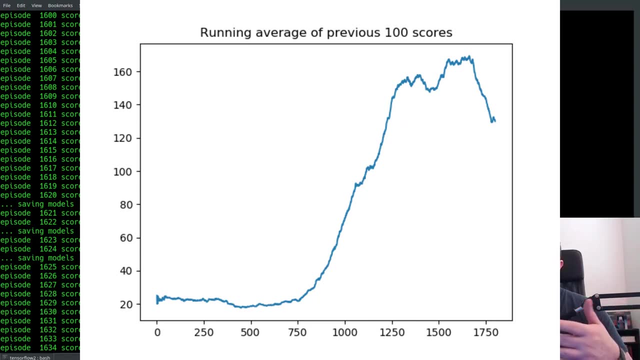 Which is almost beating the environment. It's pretty close. If you take a look at the learning plot here, You can see that it has an overall, overall upward trend and it's linear. And the reason I don't let it continue is because, as I alluded to in the lecture, 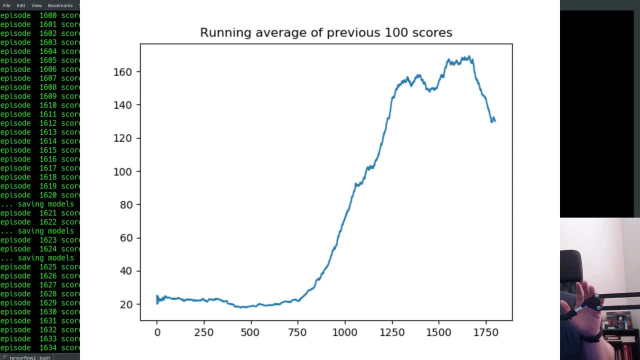 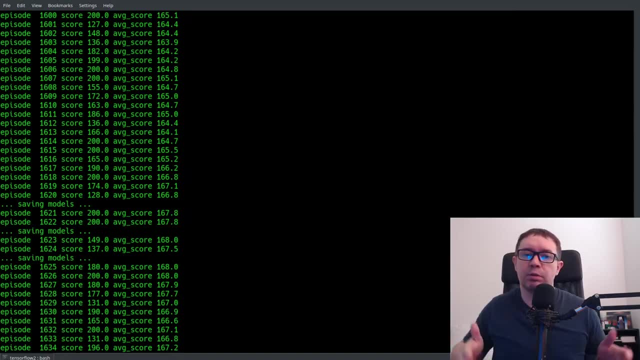 These models are very Brittle, and so sometimes you can get on a very narrow Slice of parameter space where your model is doing well, and any small step out of that range blows up the model. one thing to fix that is replay memory as you get a broader sampling of. 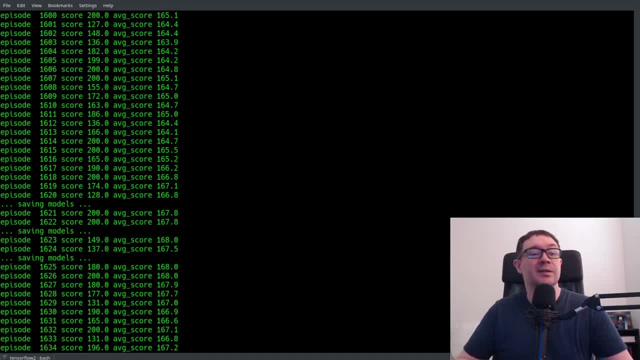 Experiences and get a little bit more stable learning. but that doesn't work. by bolting it directly onto actor critic methods- At least from my experience, I've tried it. I have a video on that. I wasn't able to get it to work. 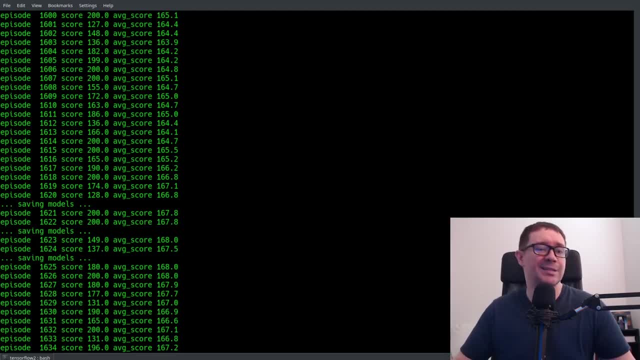 Maybe some of you can. that would be fantastic If you could, but in my case I didn't get it to work. I thought it would work. It does not and in fact there's a whole separate algorithm called actor critic with experience replay that deals with bolting experience replay on to vanilla. 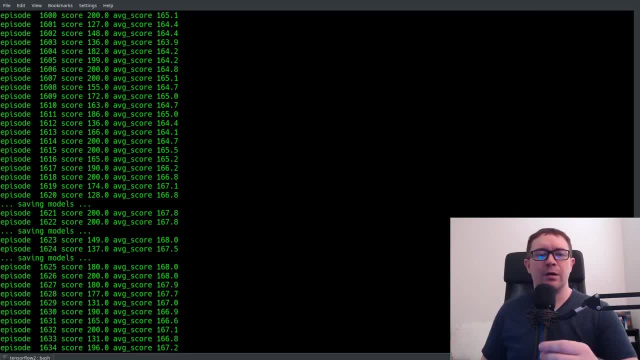 Actor critic methods, so I hope this was helpful. It's pretty hard to give a really solid overview in like a 30- 40 minute YouTube video, but it Serves to illustrate some of the finer points of actor critic methods and some of the foundational points of deep reinforcement learning in general. 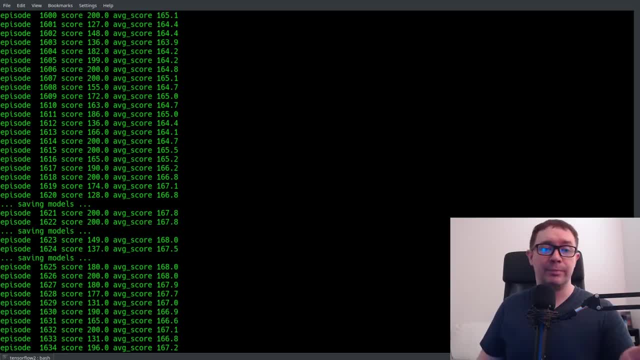 And my courses, I go into much more depth and, in particular, I show you how to actually read papers, how to turn papers into Code- a useful skill It's really hard to find anywhere else on YouTube or udemy. So if you like the content, make sure to leave a like. subscribe, if you haven't already. 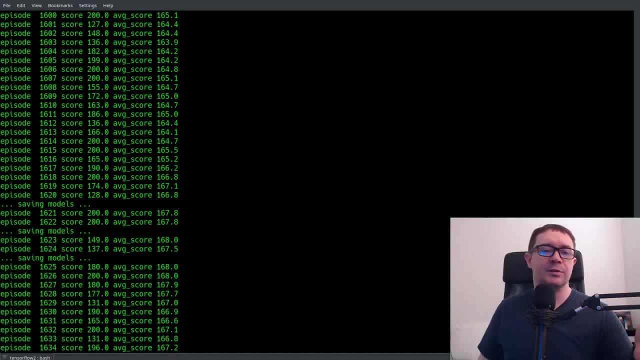 And leave a comment down below with any questions, comments, criticisms, concerns, and I will see you in the next video. Really quick, before we do, let's check in on the other terminal to make sure it's actually learning. So here is the output and you can see. 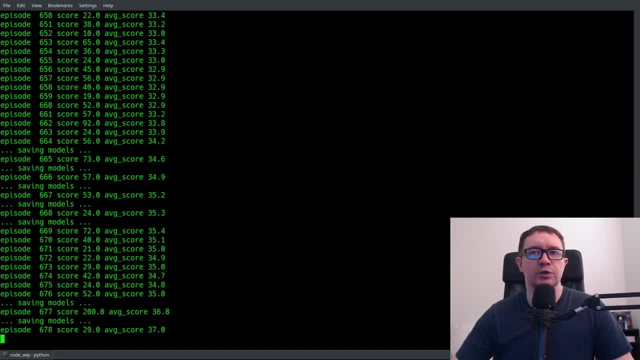 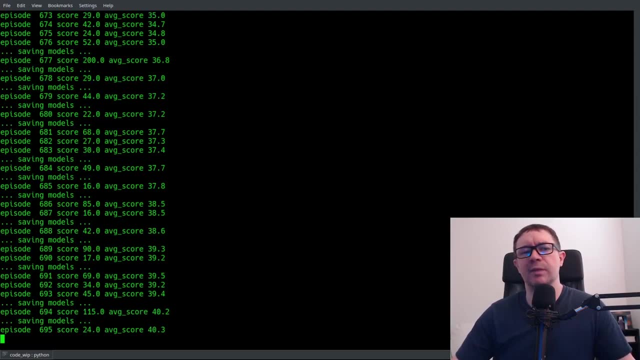 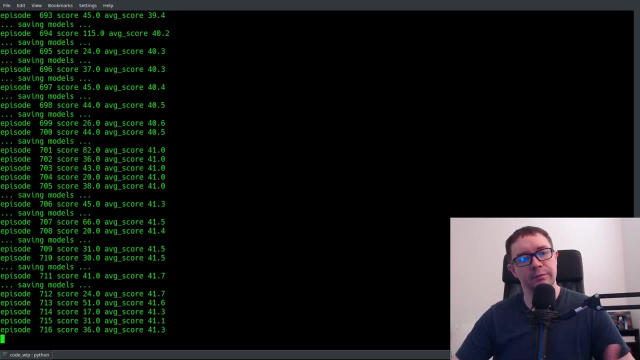 As it's going along, it is saving some models and the score is generally trending upward over time, And that's why you get the saving models, because the score is best in the last best score. So we didn't make any fundamental errors in our code. If it doesn't achieve the same result, that isn't entirely surprising, because there is a significant amount of run-to-run variation. 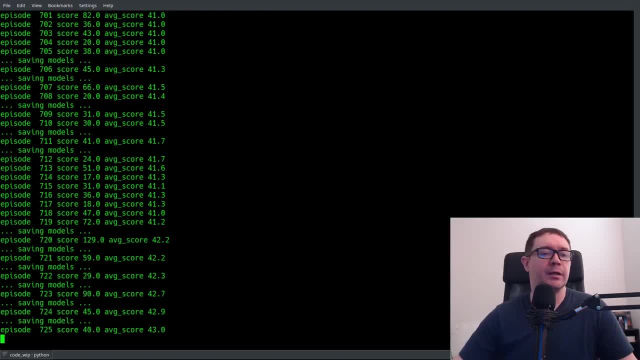 but The code is functional. What's up on my github? if you want to go ahead, check it out. I'll leave it a link in the description. See you in the next one.